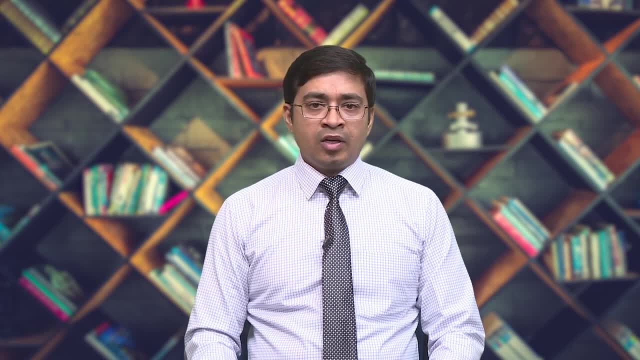 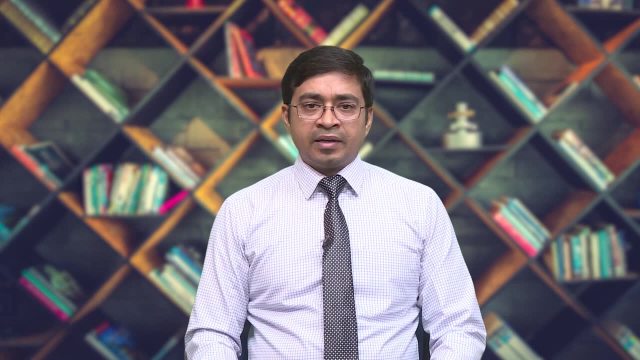 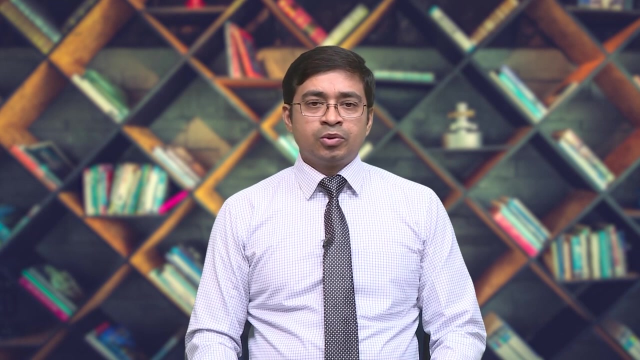 And provide an important way to understand very complex systems Such as networks that provide biology in terms of the various entities that exist and their relationship. Graphs are essentially the mathematical formalisms that are used to study networks, But the two terms are invariably used interchangeably. 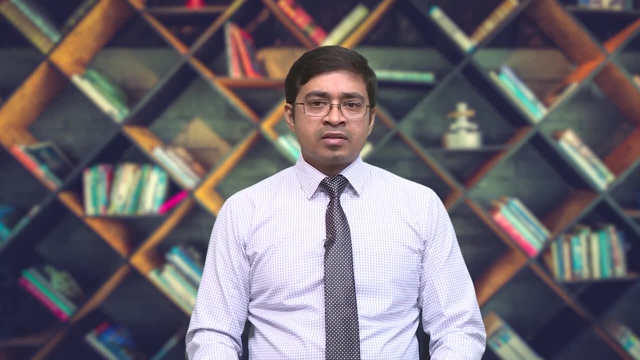 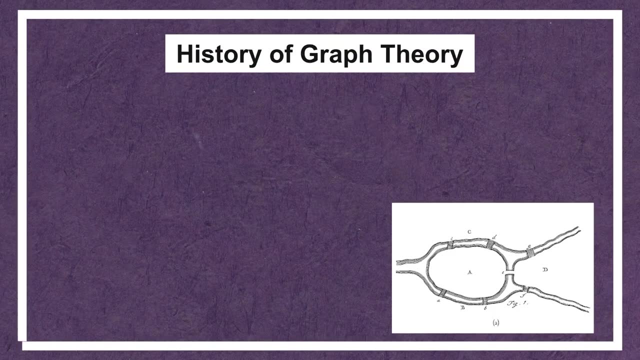 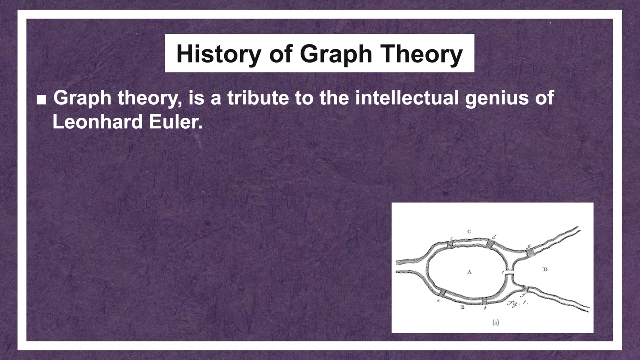 Before moving into the details graph theory, let us discuss about its history. How did this concept emerge in the history of science, The history of graph theory? Graph theory has a very interesting historical origin And, like many other mathematical concepts, it is a tribute to an intellectual genius of Leonhard Euler. 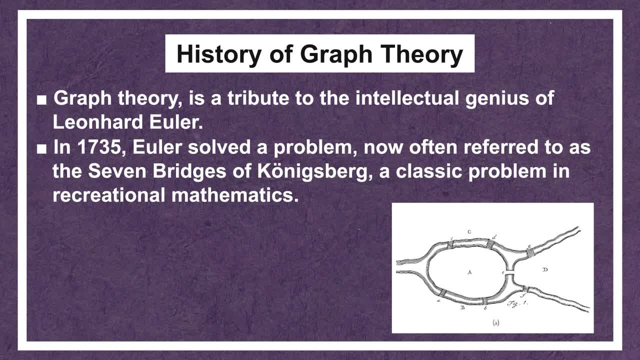 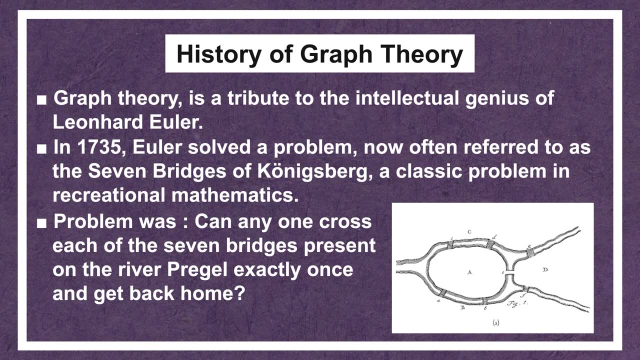 In 1735, Euler solved a problem now often referred as the Seven Bridges of Konigsberg, A classical problem in recreational mathematics. The residence of the city of Konigsberg- presently it is known as a killing guard in Russia- had an interesting thought. 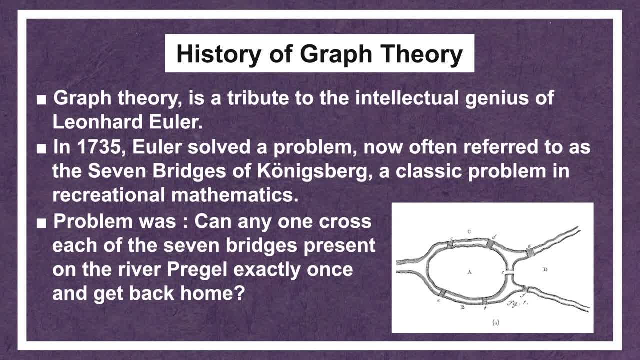 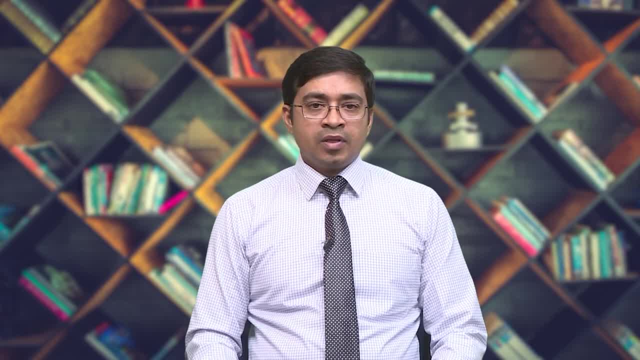 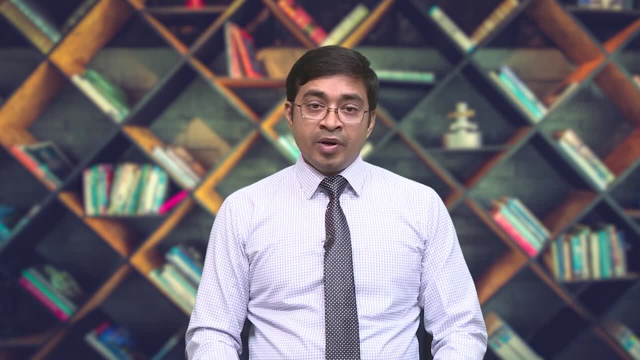 As to whether they could set out from their homes, cross each of the seven bridges on the river exactly once And get back to home. This question is so well, but seemed to be worthy of attention in the neither geometry nor algebra, nor even the art of counting was sufficient to solve it. 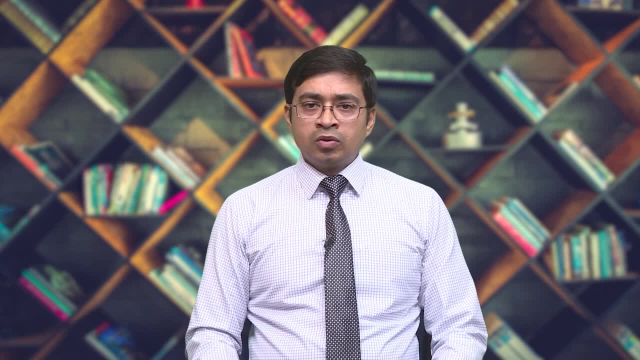 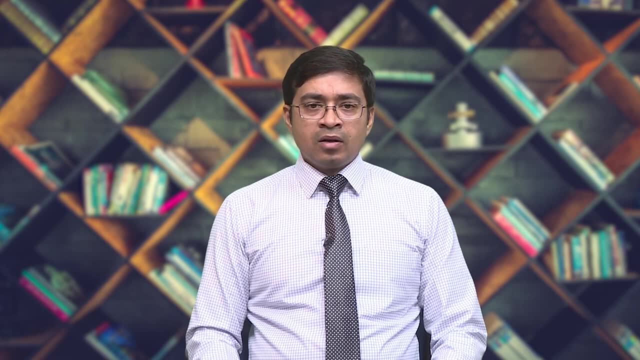 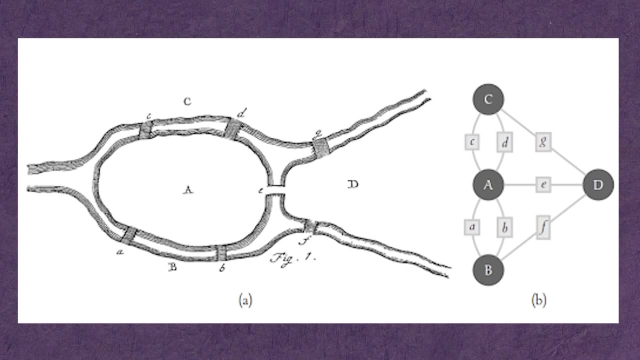 Euler, of course, solved this problem. Euler, of course, solved this problem in a negative aspect, Showing that no such walk exists, So nobody can cross the river by crossing each once Figure A represents in this slide. so Euler's sketch derived from the map of the city. 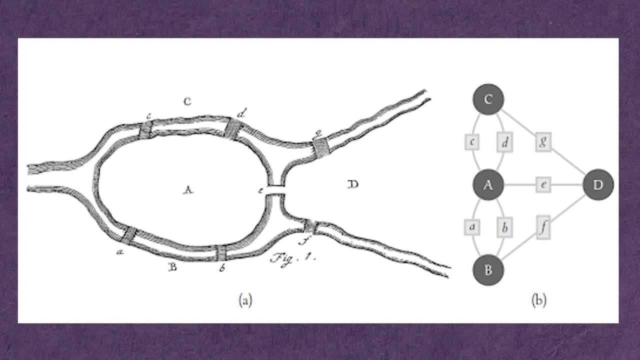 While figure B is the first graph that was ever created, Note the mapping of nodes and edges as land masses and the corresponding bridges. The graph he made in 1735 is denoted the land masses by capital letters A to D And seven bridges on the river Pregel represented by small letter A to G, as shown in figure. 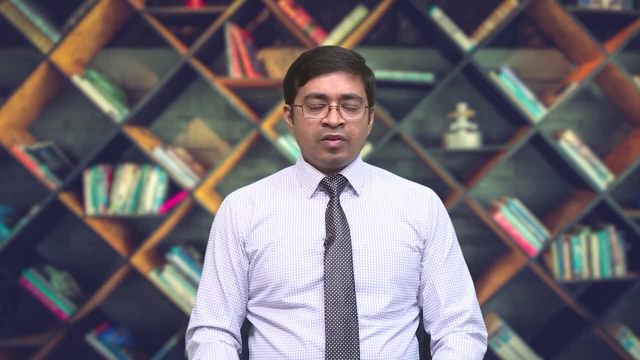 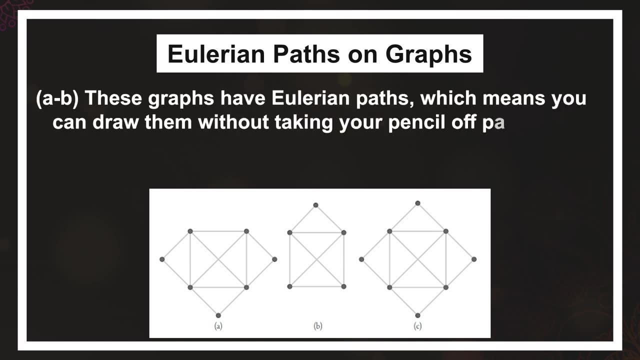 However, it is not a simple graph, given that it has a parallel edges running between the same pairs of vertices, But path that began and ended the same vertex of a graph, passing through every single edge in the graph exactly once, Are now called Eulerian cycle. 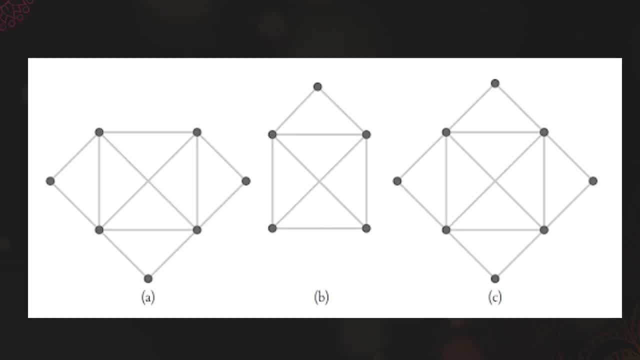 In honor of his solution of Euler. Figure A, B and C present in this slide show some example of graph with and without Eulerian path. Finding Eulerian path in graph has more far-reaching consequences than solving the recreational mathematics problem. Figure A and B have Eulerian path. 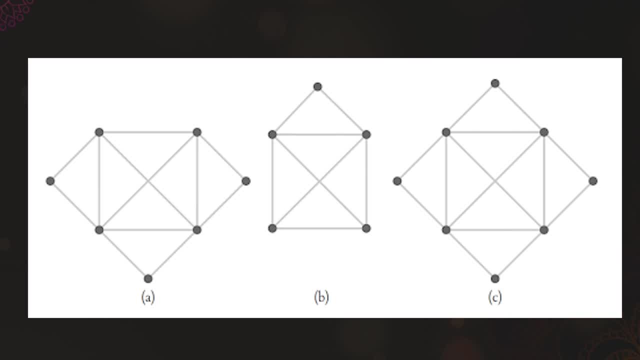 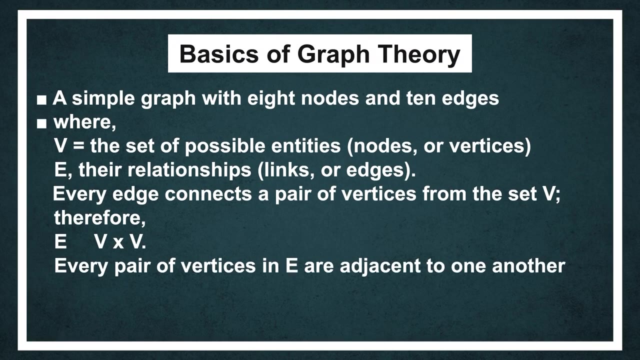 Which means you can draw them without taking your pencil or paper, passing through all edges exactly once, While in figure C this graph does not have an Euler path. Let's discuss about some basics of graph theory. Formally, a graph which can be represented by capital G is denoted as a set of V and E. 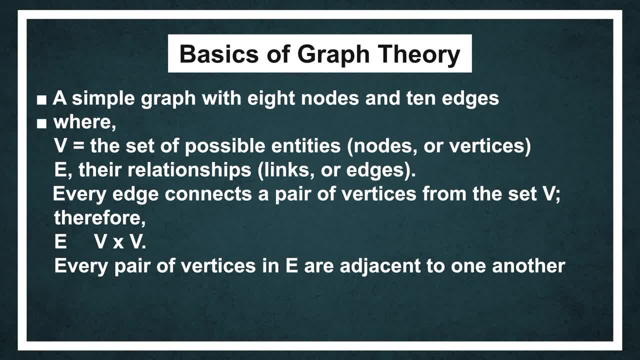 where V represent the set of possible entities, namely nodes and vertices, And set of E. it is relationship of the all entities. It is also known as link or edges. Every edge connects a pair of vertices from the set V. Every pair of vertices in E are adjacent to one and another. 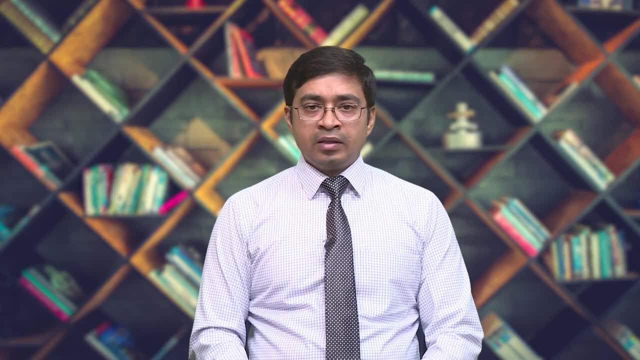 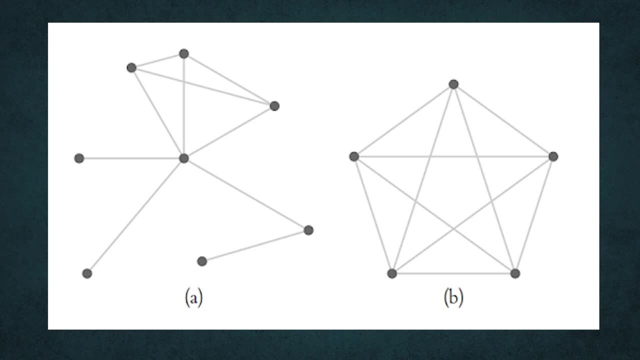 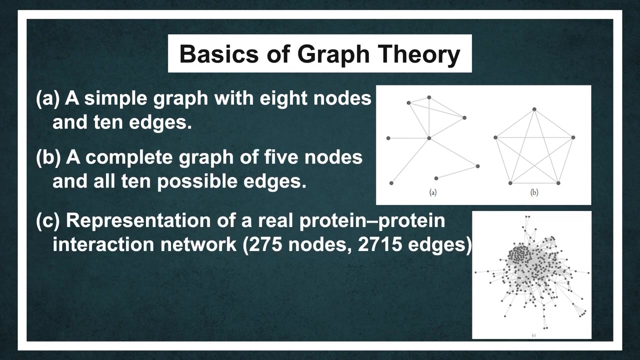 Some simple illustration graph are shown in figure. the coming slides Here. in figure A, a simple graph with 8 nodes and 10 edges. Figure B represent complete graph having 5 nodes and 10 possible edges, And figure C, which is a snapshot of real protein-protein interaction network having 275 nodes and 2715 edges. 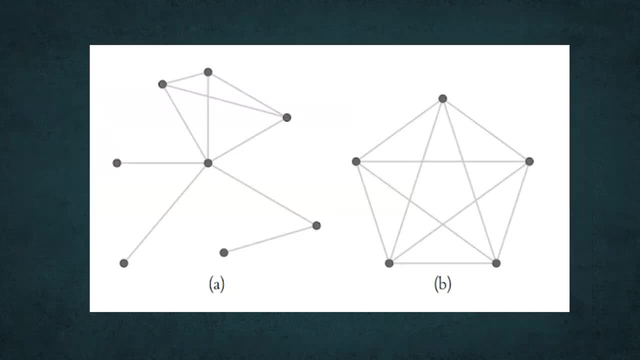 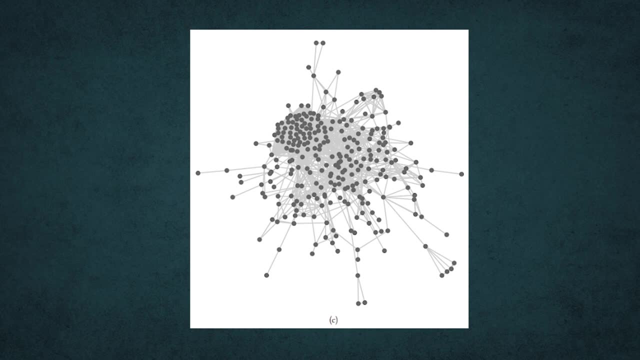 Every node represent a protein in the bacterial mycoplasma genitalium from the string database version 10.5.. Only functional association and interaction with the confidence of 900 and above from the single largest component of the graph are shown in the figure C. 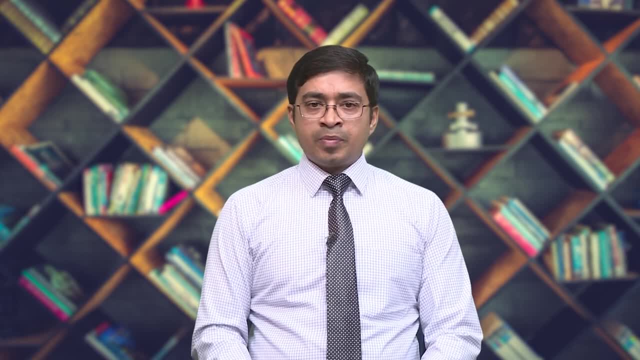 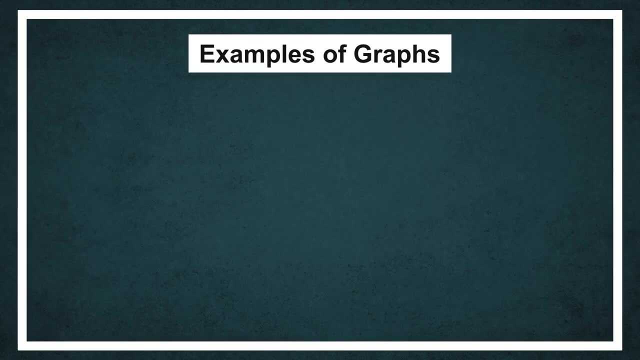 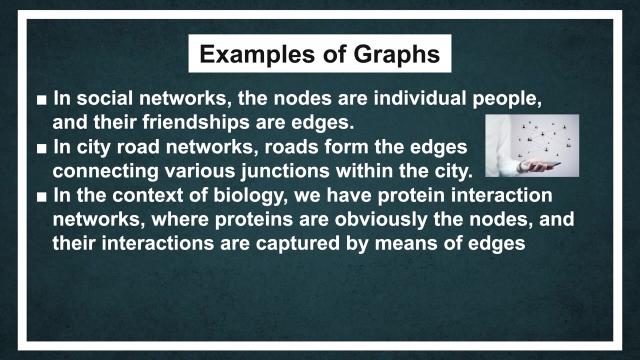 So let's have a look on certain examples of graph To fix ideas. let us review a few examples of graph. Every graph, as discussed above, needs to be described by a set of node, or vertices, and a set of edges. In social network, nodes are edges. 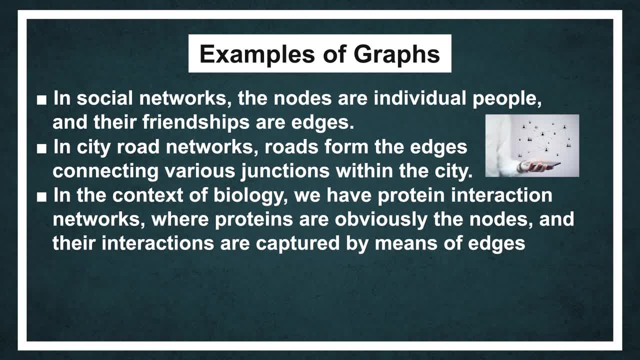 Individual people and their friendships are edges In city-road networks. roads form the edges connecting various junctions within the city. In the context of biology, we have protein interaction network, where protein are obviously the nodes and their interactions are captured by means of edges. 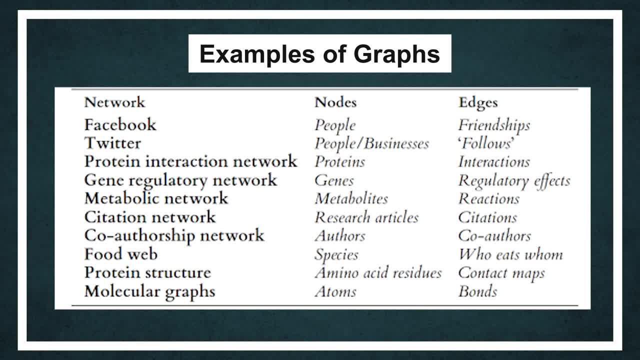 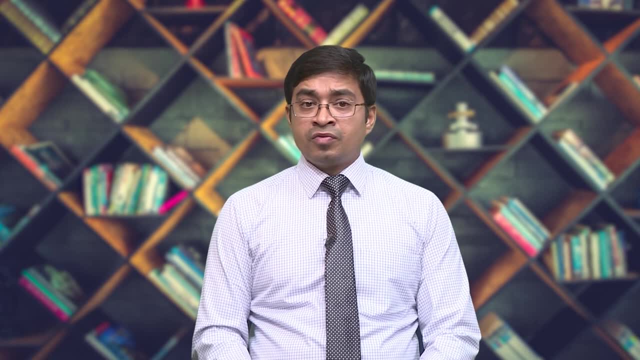 List. a few networks are provided in given table, indicating what their nodes and edges typically describe. So next question come in the mind is why such graph are important. What are the importance of these graphs? So graphs are useful to answer many interesting question about different type of system. 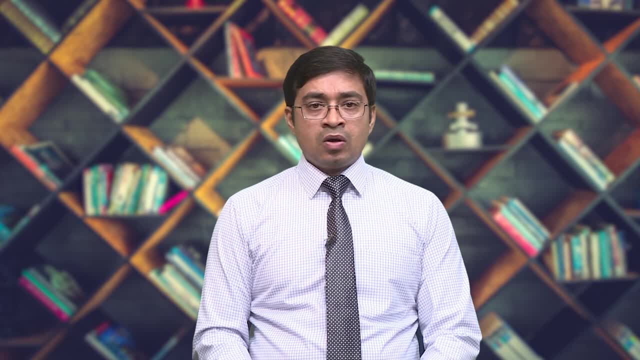 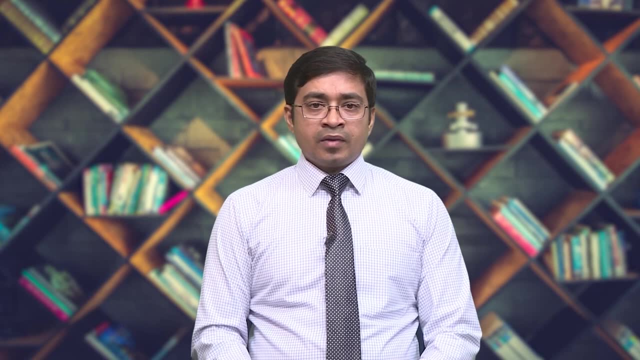 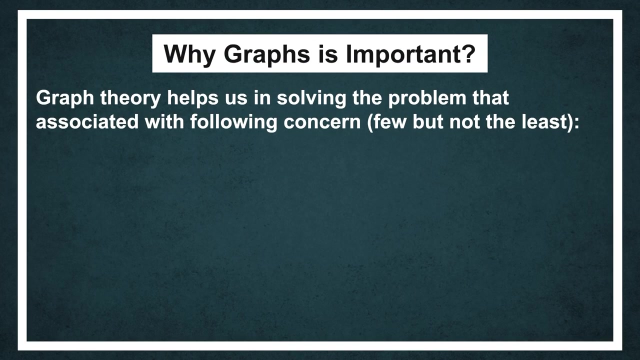 For instance, social network analysis, or sociometry as it was originally called, is dated to the early 1930s. In the context of social network, many interesting questions have been asked, of graph, For example. first question: do I know someone who know someone who know? X is an example of existence of path problem. 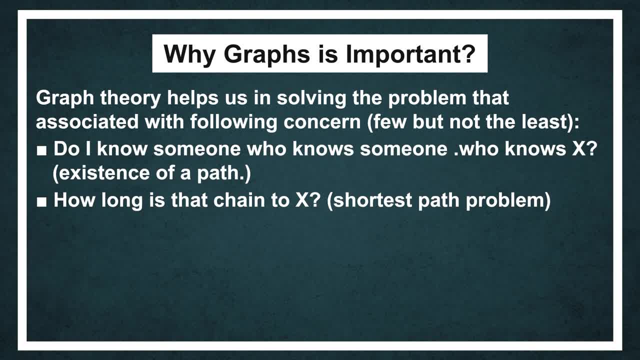 Another question: how long is that chain to X? is a kind of shortest path problem. Another one is everyone in the world connected to one another is a kind of identifying connected components kind of problem. Next question was kind of who has the most friend or who is the most influential person? 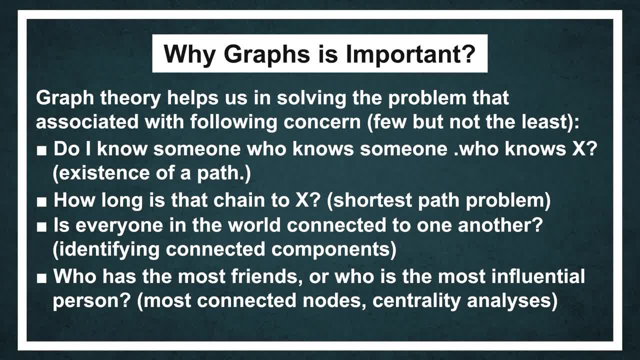 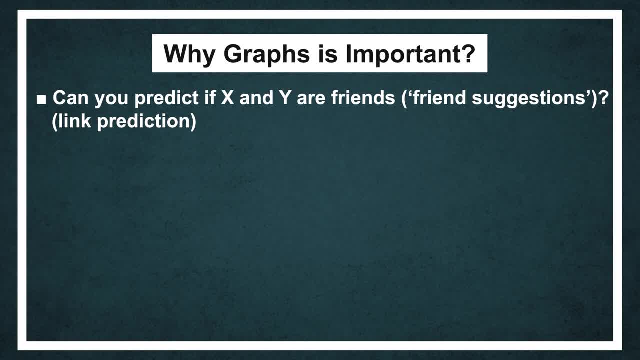 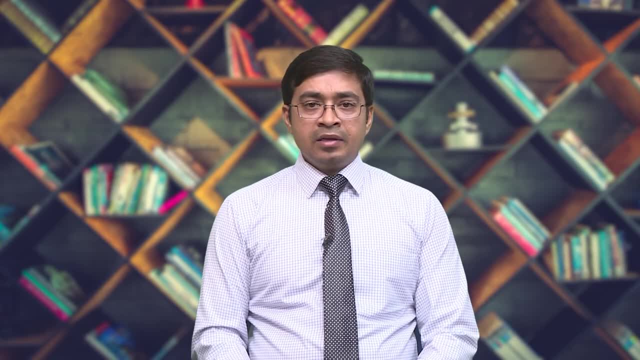 It is a concern of most connected nodes, centrality analysis kind of problem. Another category of problem is we can say: can you predict if X and Y are friends? Friends suggestion can be give. it is kind of link prediction problem. Interestingly, in a very similar way, question are often of interest in the context of biological network. 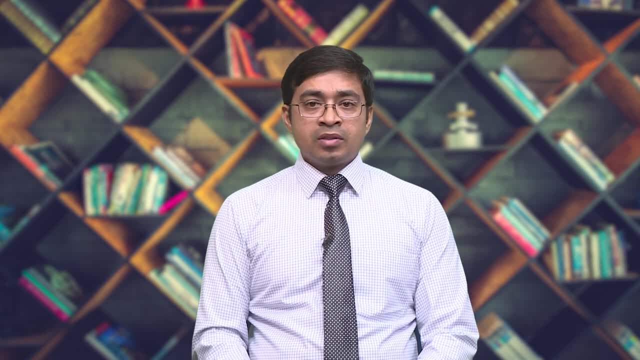 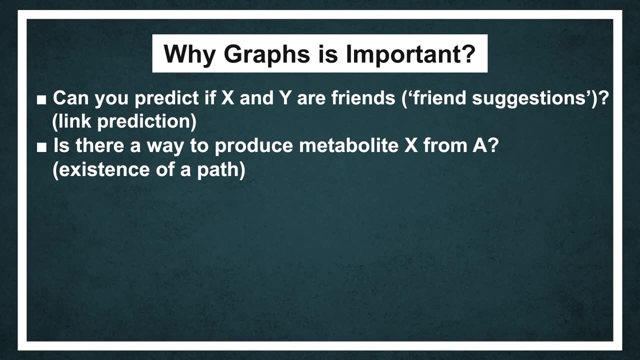 And can be address using pretty much the same graph algorithm. Question one with respect to biological network: is there a way to produce metabolite X from A? Second question is: how long is the optimal chain from X to A? Another category are all protein connected to others by a path. 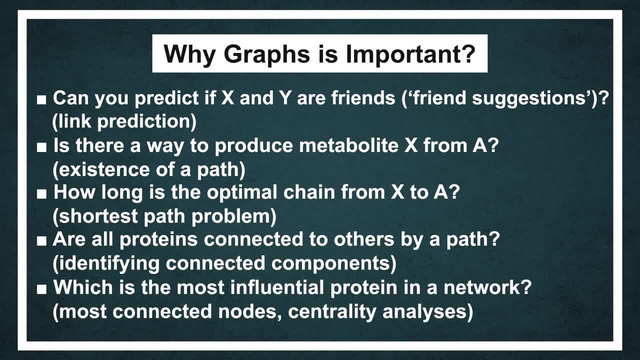 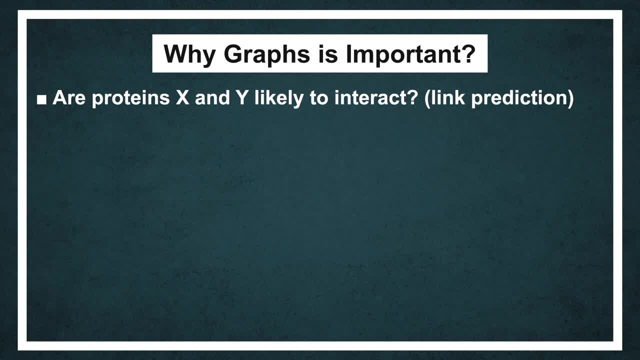 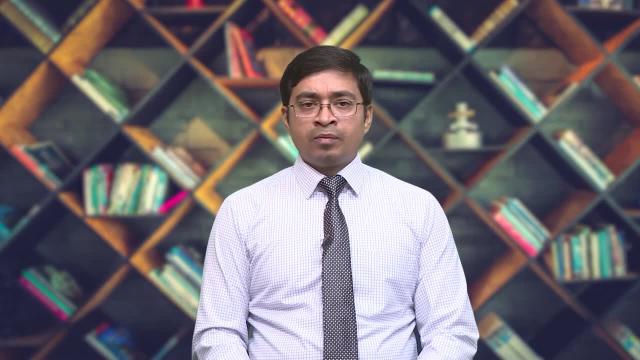 The fourth kind of question: which is the most influential protein in the world In the network? And fifth question is kind of: are protein X and Y likely to interact each other? So such kind of problem can be solved with the Hap-Hop graph theory. 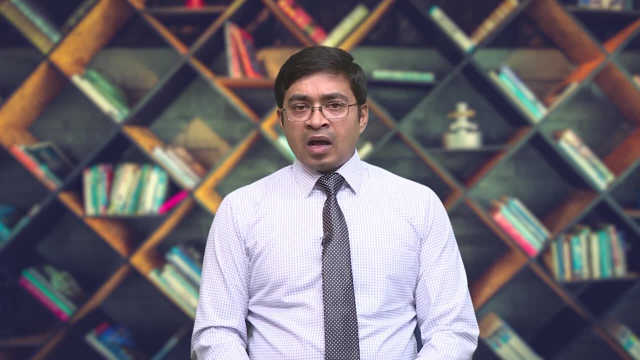 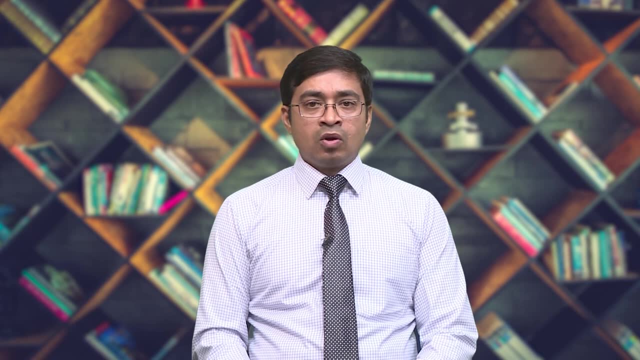 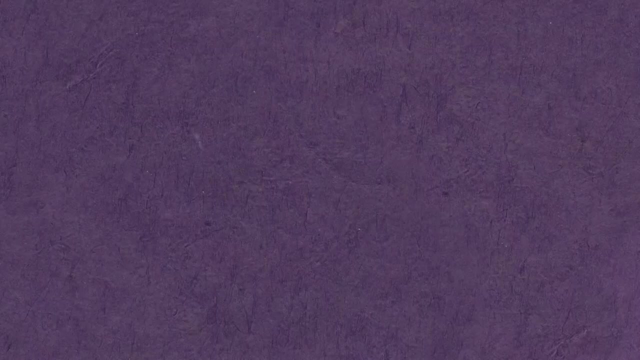 So the graph can be classified into different types based on the nature of connections, the strength of the connections and so on. Here we will review some of these basic concepts. Total: there are twelve types of graphs, Namely simple versus non-simple graph. 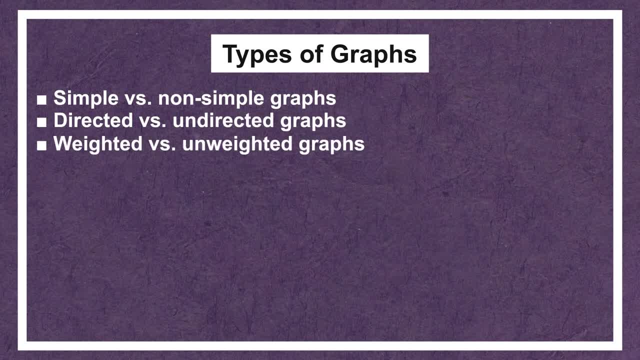 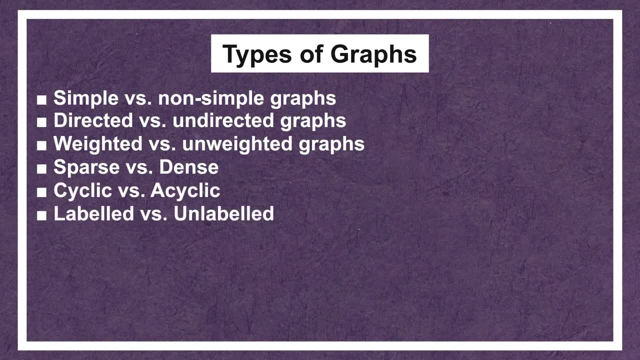 Directed versus non-directed graph. Weighted versus unweighted graph. Spurs versus dense graph. Cyclic versus acyclic graph. Labeled versus unlabeled graph. Isomorphic versus non-isomorphic graph. Biparatite graph. Implicit graph- Regular graph. 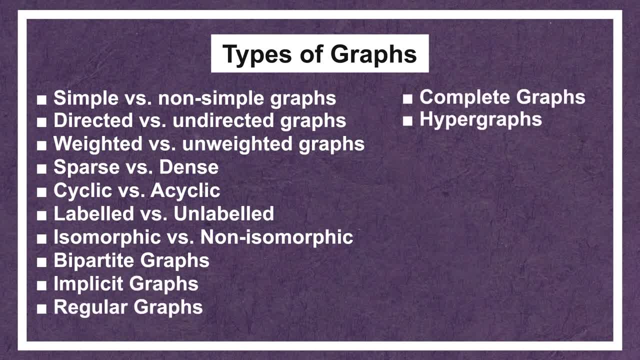 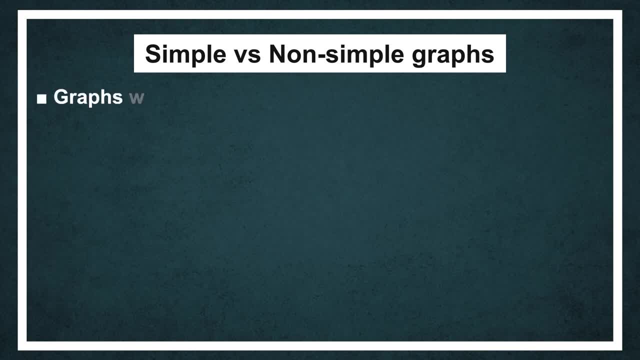 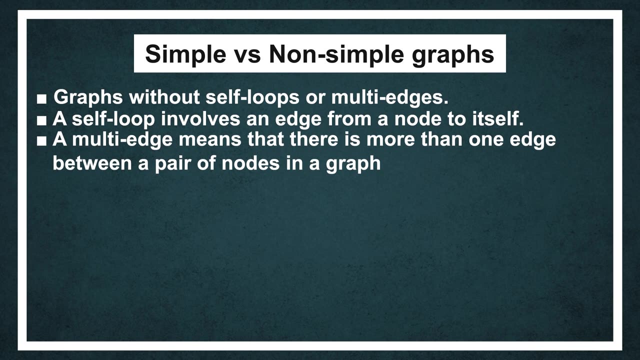 Complete graph And finally, hypergraphs. Let's discuss one by one: So simple versus non-isomorphic graph. A simple graph or graph without self-loop or multi-ages. A self-loop involves an edge from a node to itself. A multi-age means that there is a more than one edge between a pair of nodes in a graph. 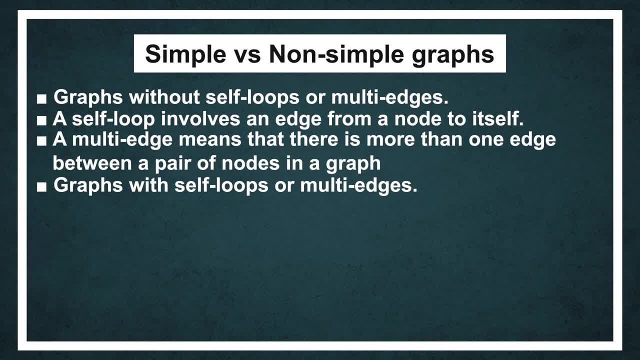 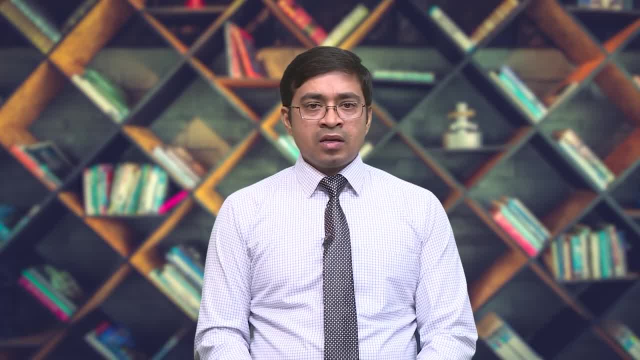 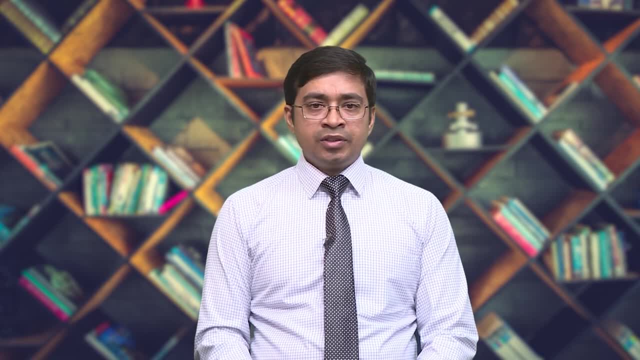 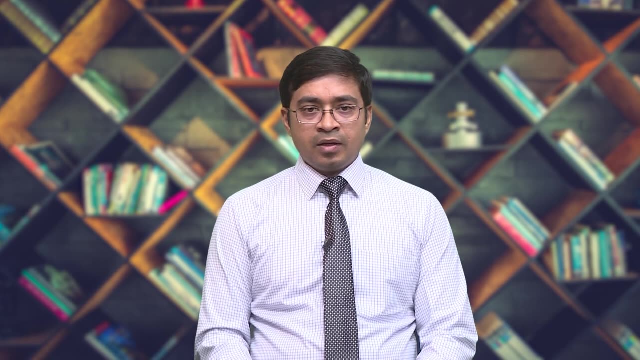 So self-loops and multi-ages necessitate special care while working with graph and graph algorithms. Simple graphs are devoid of such structure. Self-loop do occurs in gene regulatory network, where a gene can inhibit its own synthesis, thus resulting in a vertex connected to itself. 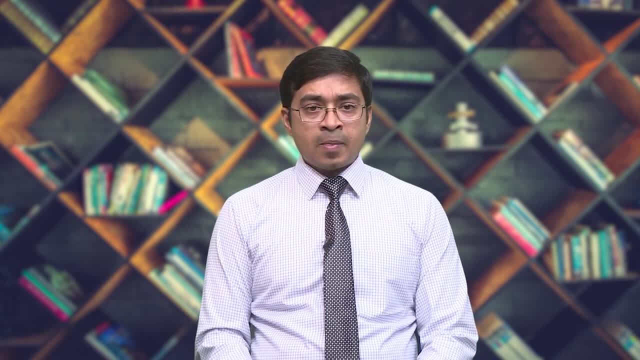 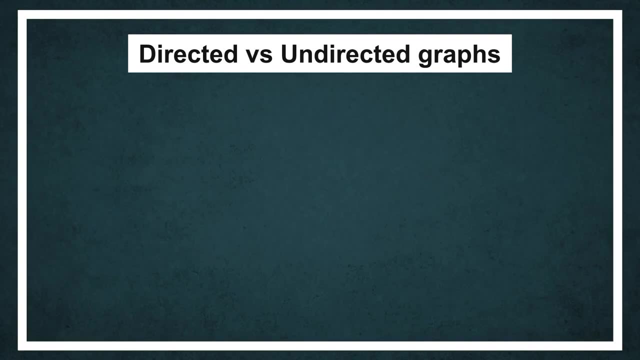 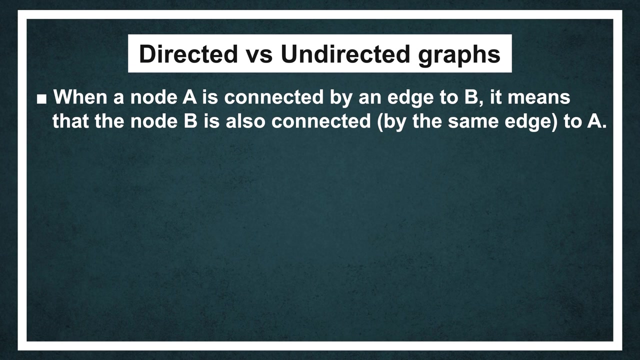 Second example of graph is directed versus undirected. Perhaps the most of important classification of graph is based on the symmetry of edges Into directed and undirected graph. Undirected graph: when a node A is connected to the node B, It means that the node B is also connected to A. 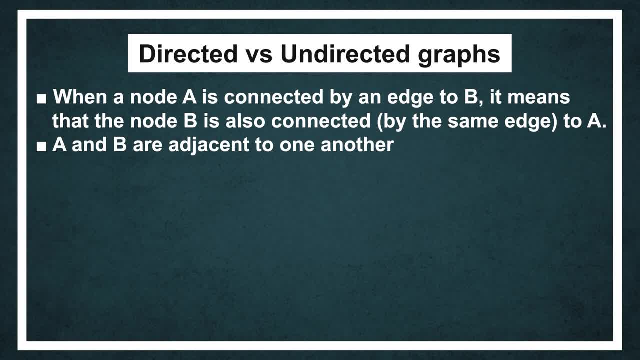 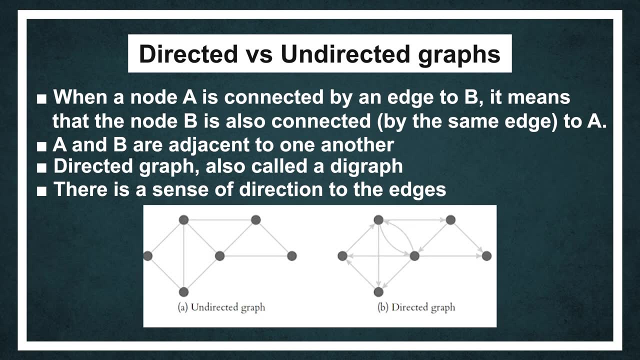 In other word, A and B are adjacent to one another. On the other hand, in a directed graph, also called a digraph, there is a sense of direction to the edges, As shown in figure A and B, While A may be connected by an edge to B. 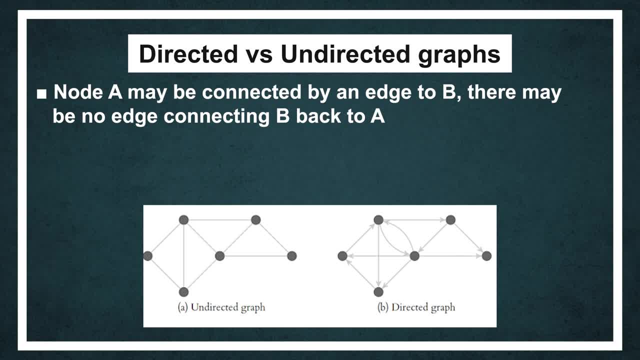 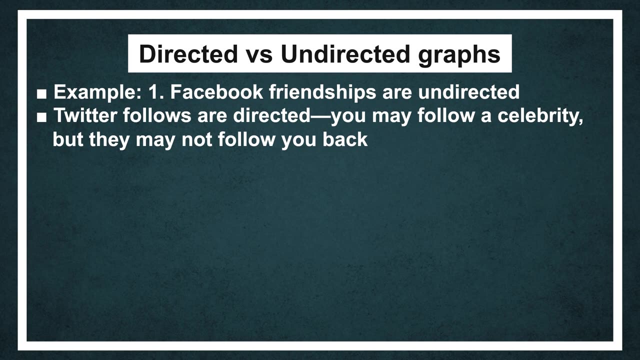 There may be no edge connecting B back to A. A classic example of directed network is that of CT roads network, With its one-way road, which will result in some pair of junction being connected only in one direction. In social network, Facebook friendships are undirected, whereas Twitter follows as a directed. 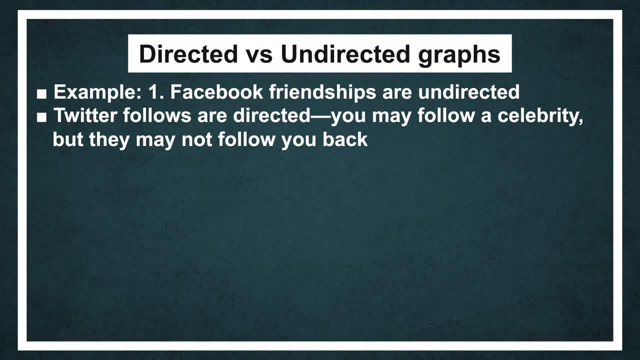 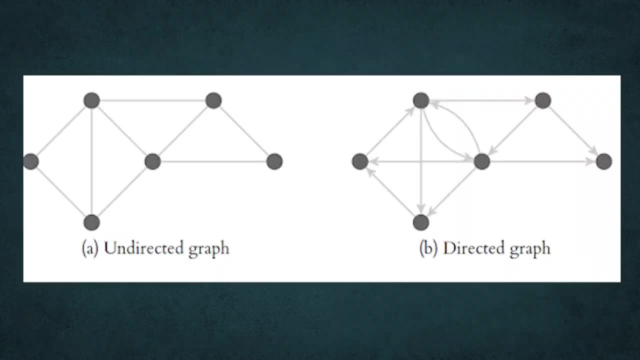 You may follow celebrity, but they may not follow you back. In the context of biology, protein interaction network are typically undirected, While gene regulatory network are directed. A gene A may activate a gene B, But gene B may have no effect on the activation or repression of a gene A. 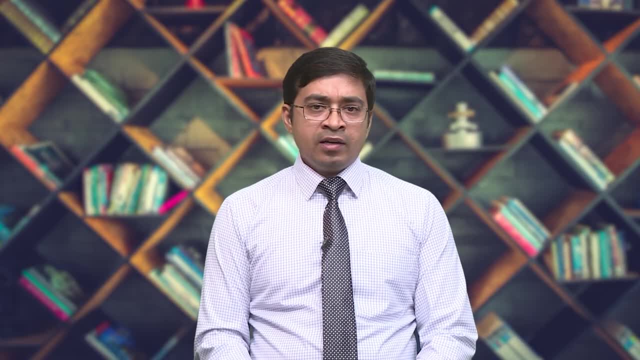 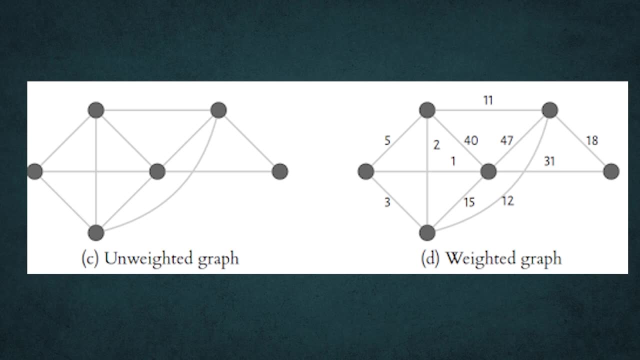 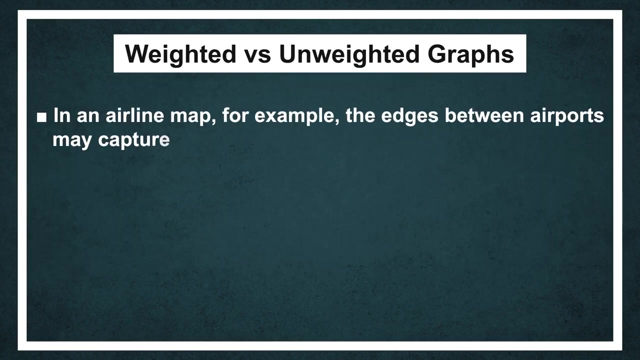 So next category of graph is weighted versus unweighted graph. The age between nodes in a graph may be associated with weight, Which typically represents some sort of cost, as shown in figure C and D. In an airline map, for an example, the edges between airport may capture distance or flight fares. 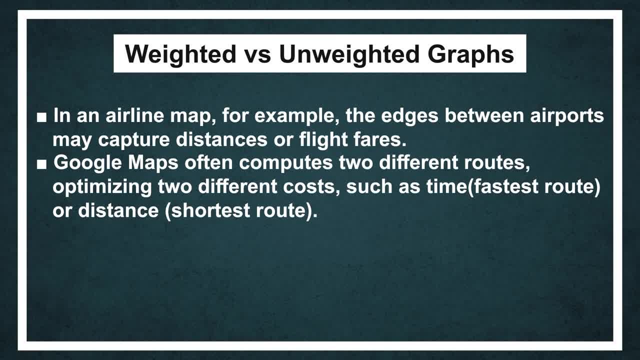 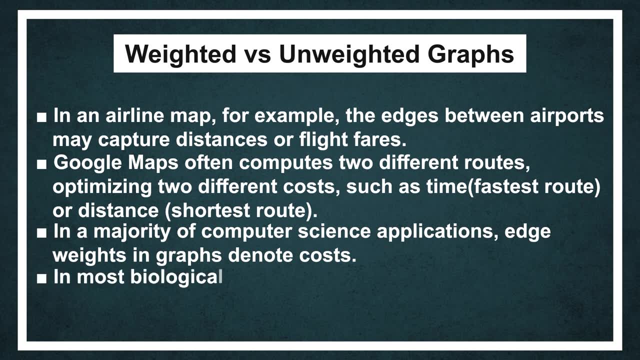 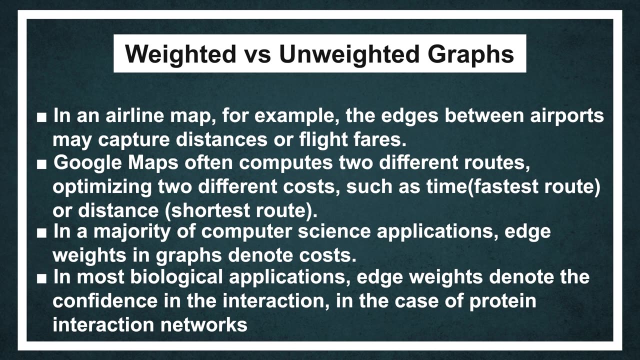 Google map often computes two different routes, optimizing two different cost, such as a time or distance. In a majority of computer science application, Age weights in a graph denote cost. In most biological application, Age weight denote the confidence in the interaction. In the case of protein interaction, network or similarity. 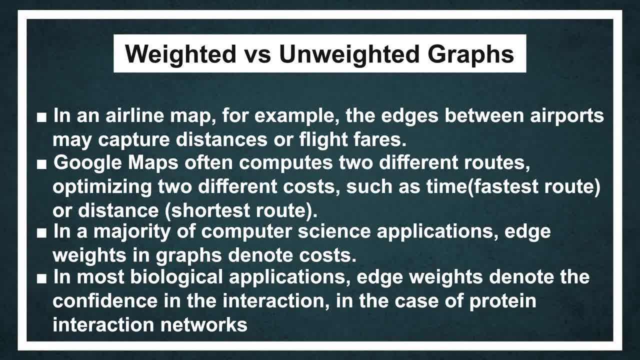 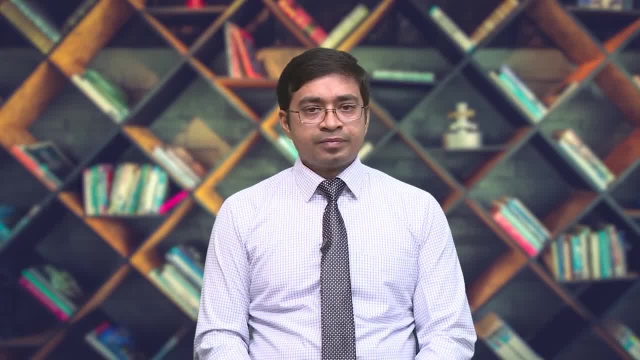 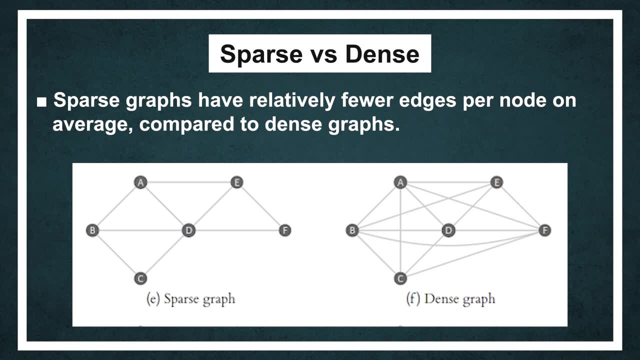 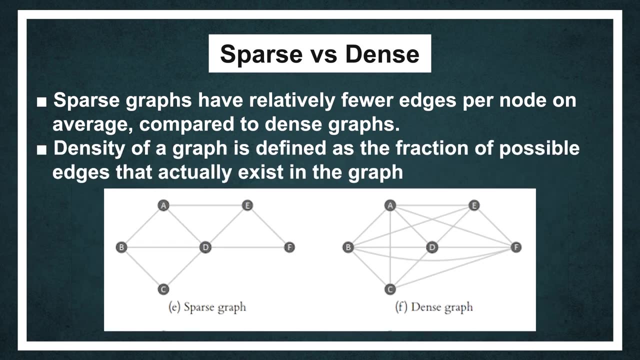 And in the case of co-expression networks. One more type of graph, known as spurs, versus dense graph. The spurs graph have relatively fewer edges per node on average, Compared to dense graph. can prefer figure E and F. Density of graph is defined as the fraction of possible edges that actually exist in the graph. 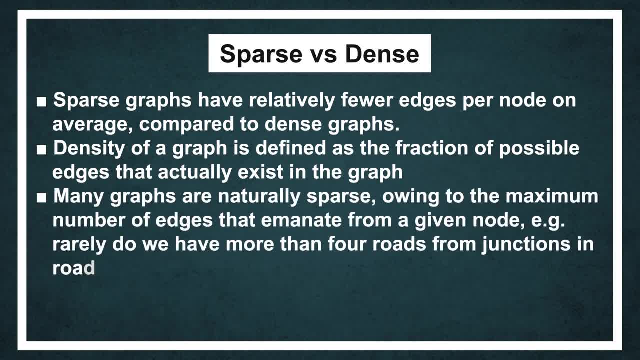 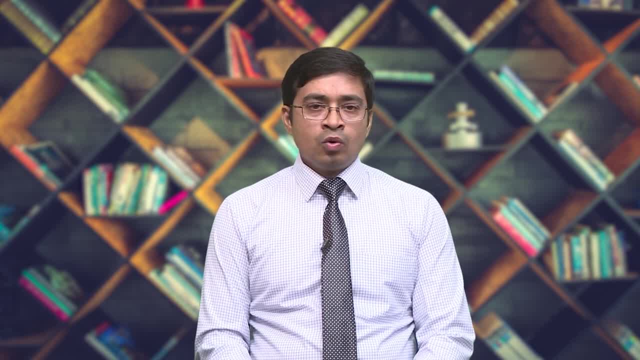 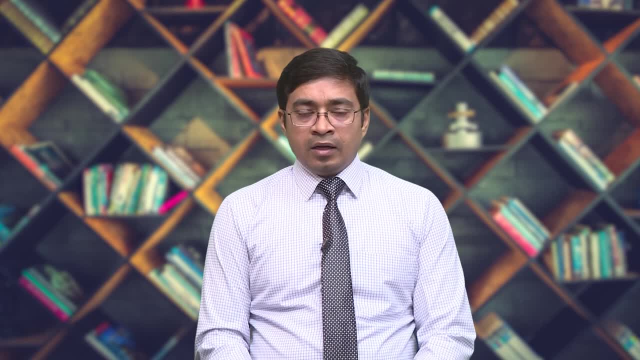 Many graphs are naturally spurs owing to the maximum number of edges that emanate from a given node. Example: rarely do we have more than four roads from junction in a road network. Most biological network are also quite spurs. type Another category of graph known as cyclic versus acyclic graph. 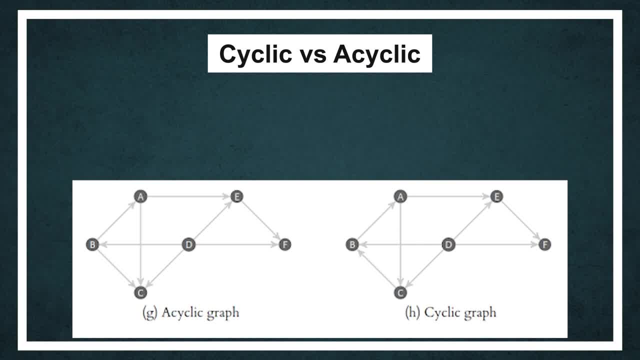 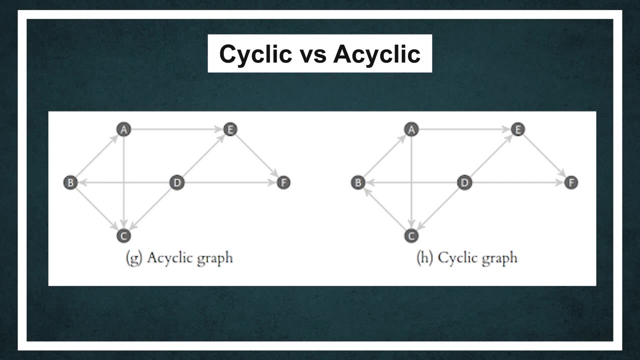 Graph can be classified as cyclic or acyclic, depending on the existence of one or more cycles. A cycle in a graph is a path from a node to itself. In the graph of figure H, there is a cycle involving node A, C and B. 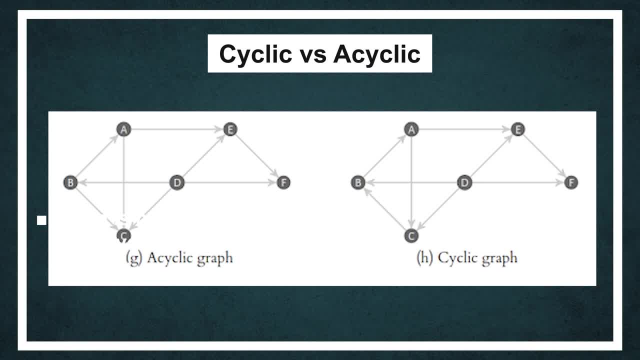 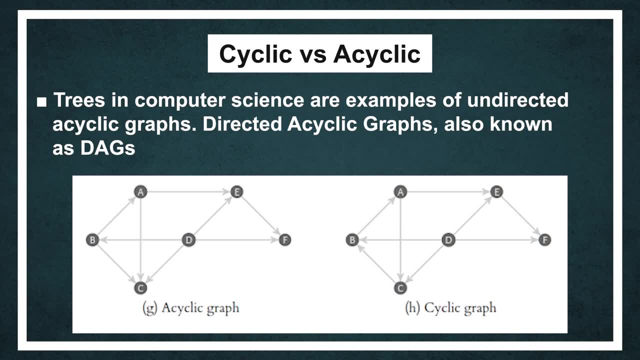 On the other hand, there is no such cycle in figure G. Trees in computer science are example of undirected acyclic graph. Directed cyclic graph, also known as DAGs, naturally arise in many scenarios, such as in scheduling problems: Labeled versus unlabeled graph. 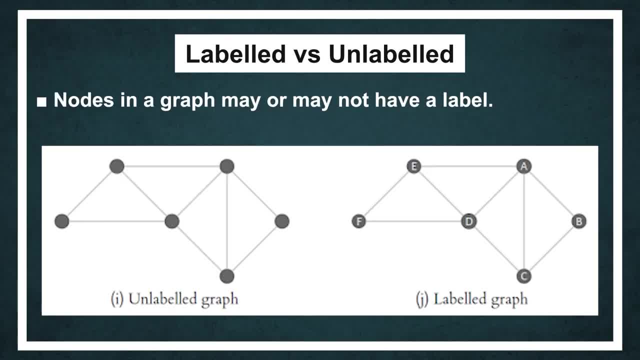 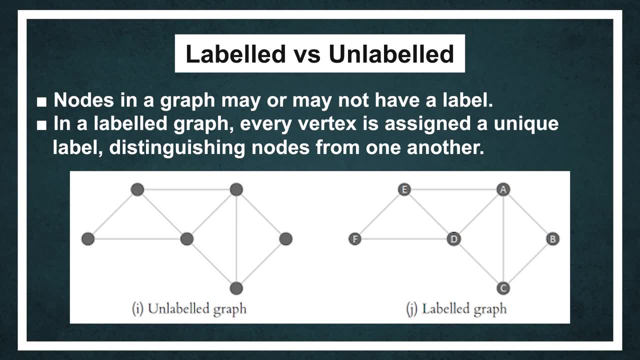 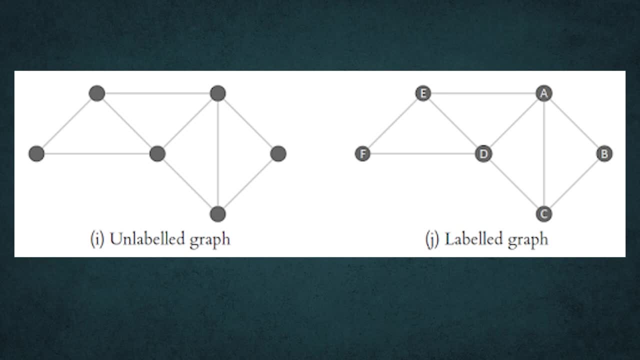 Here nodes in a graph may or may not have a label. In a labeled graph every vertex is assigned a unique label distinguishing nodes from one another. Here figure I is an unlabeled graph, while figure J represent a labeled graph. Real word graph are naturally labeled. 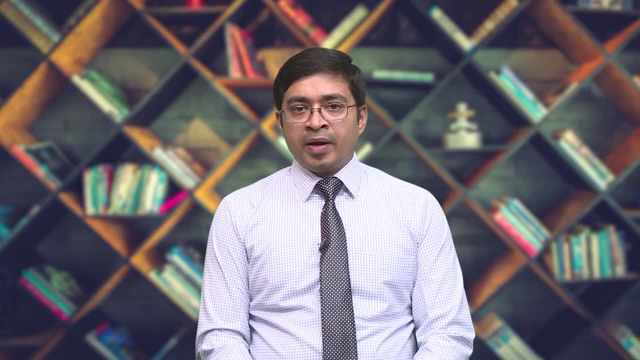 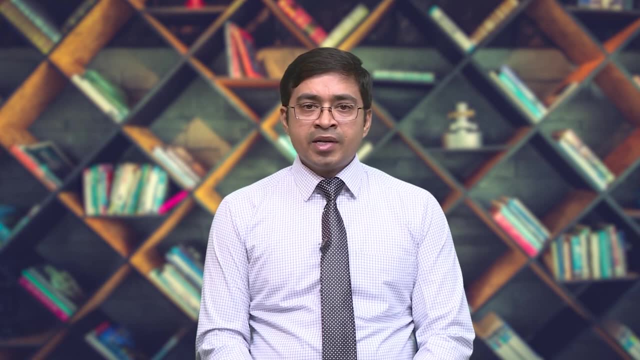 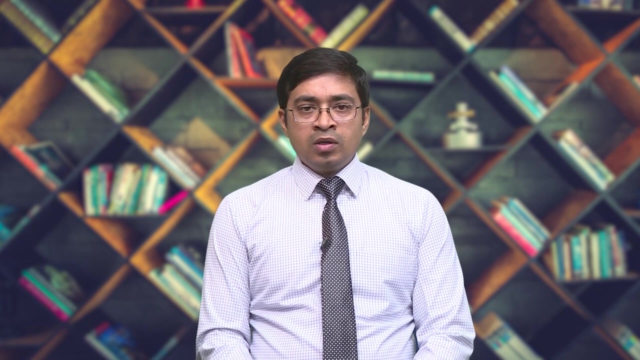 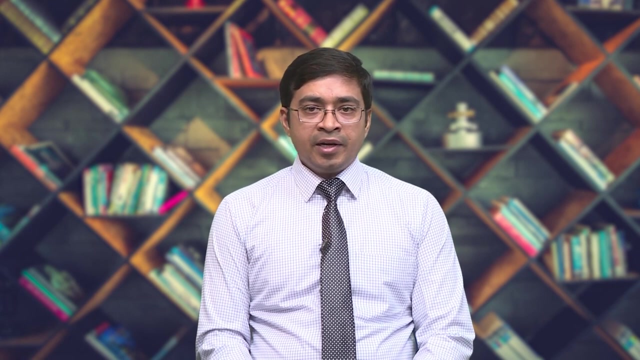 Example, using protein names or metabolite names. In some applications the label need not to be unique, like while representing molecule as graph, with nodes being labeled by atom Labels are typically ignored while testing for graph Isomorphism to determine if two graphs are topologically identical, if we ignore node labels. 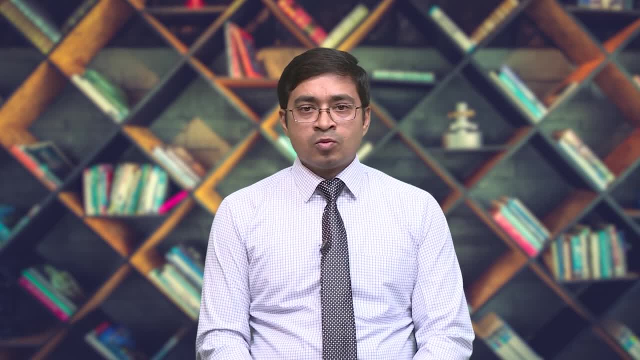 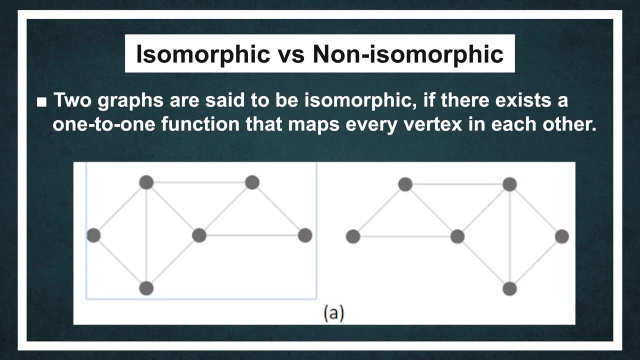 Next type of graph is known as isomorphic versus non-isomorphic graph. Two graph, named G1 and G2, are said to be isomorphic. if there exist are one-to-one functions that map every vertex in graph 1 and to every vertex in graph 2.. 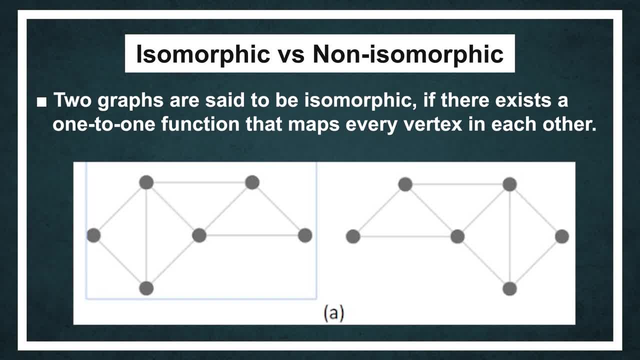 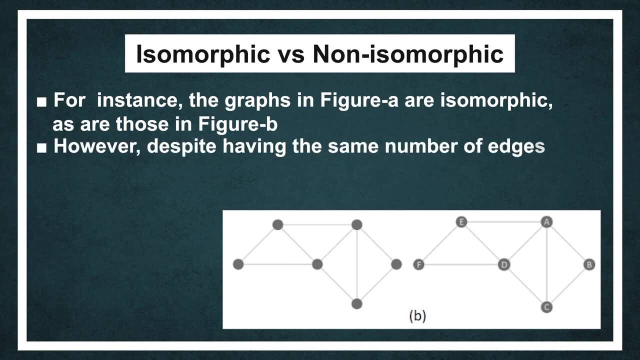 Such that two vertices in graph 1 are connected by an edge if, and only if, their corresponding vertices in graph 2 are connected by an edge. For instance, the graph in figure A and B are isomorphic. However, despite having the same number of edges and nodes, the graph in figure C are not isomorphic. 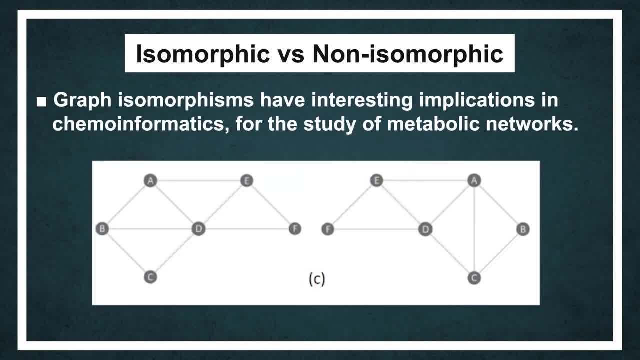 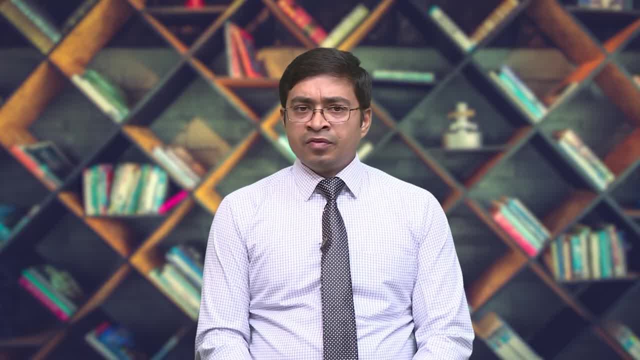 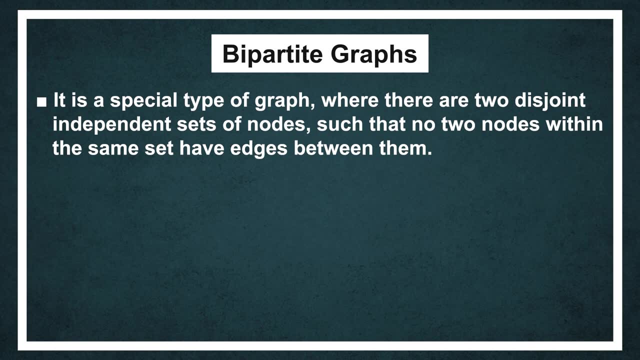 Graph isomorphism have interesting implications in chemo-integration. Another graph that are known as bipartite graph. A bipartite graph is a spatial type of graph where there are two disjoints, independent set of nodes, such that no two nodes within the same set have edges between them. 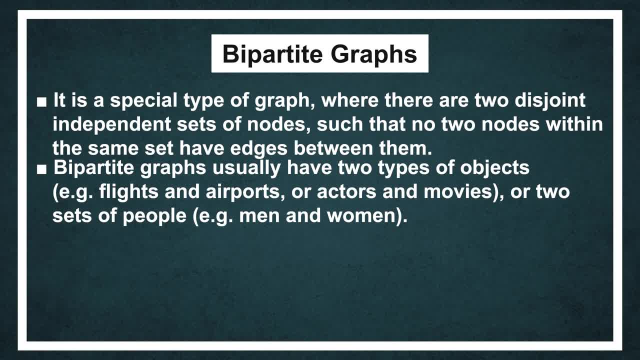 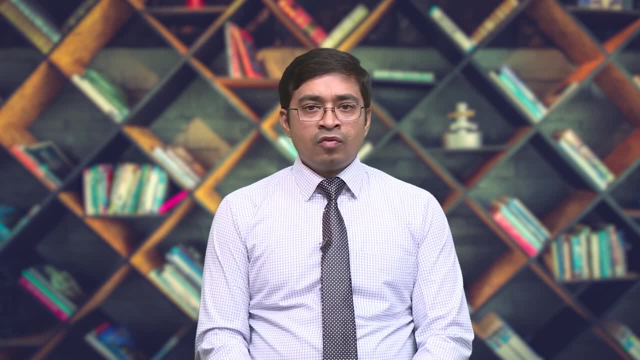 Bipartite graph arise naturally in scenario where there are two types of objects, like flights and airports, Or actor and movies, Or two set of peoples, like men or women. Film actor networks are bipartite where the two set of nodes represent actors and movies. 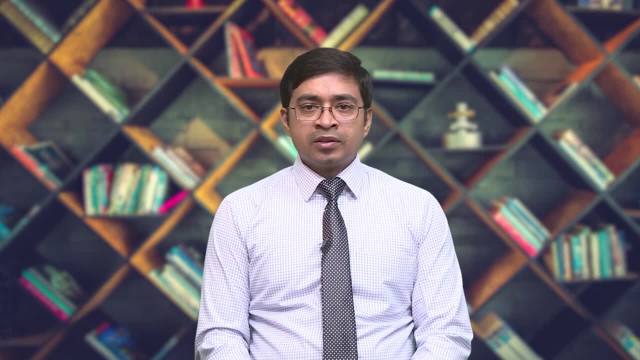 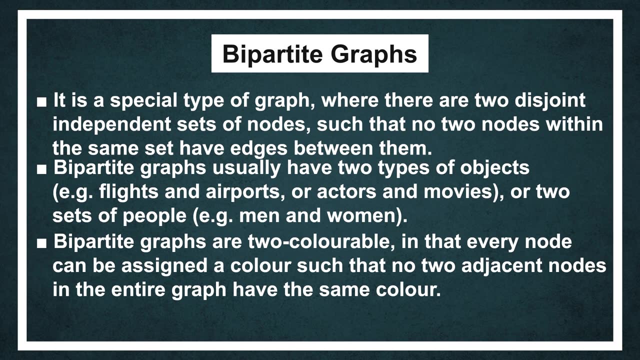 And the edges connected actors to the movie they started. in Bipartite graph are two colorable. In that every node can be assigned a unique color such that no two adjacent nodes in the entire graph can be assigned. In that every node can be assigned a unique color such that no two adjacent nodes in the entire graph can be assigned. 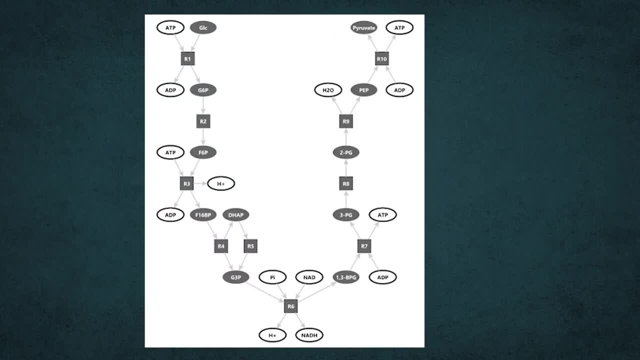 In that every node can be assigned a unique color, such that no two adjacent nodes in the entire graph can be assigned. It is also helpful to think of, in the term of shapes, A graph of square and ellipsis, Where no ellipsis is adjacent to each other. 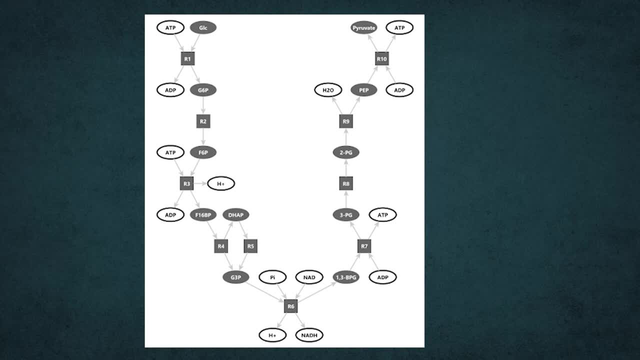 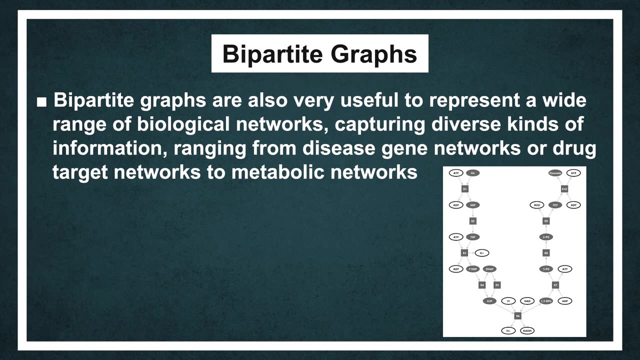 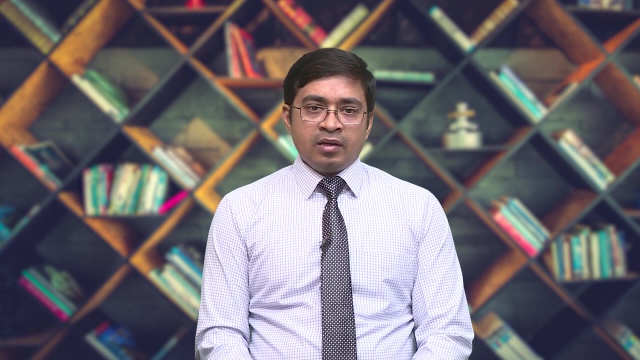 And no square is connected to another. squares Bipartite graph are also very useful to represent a wide range of biological networks Capturing diverse kind of information, Ranging from disease Gene network Or drug target network To metabolic network. Another type of graph is known as implicit graph. 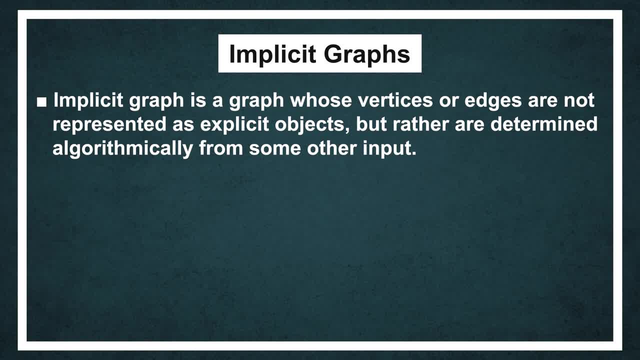 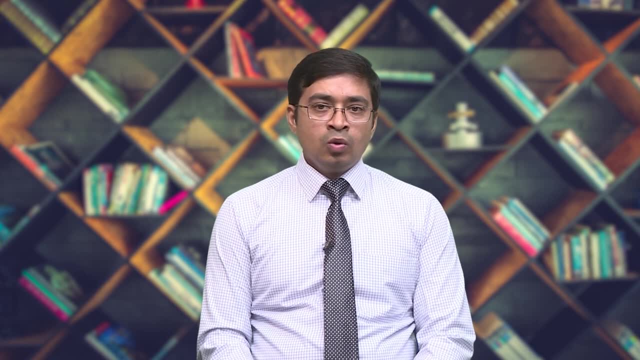 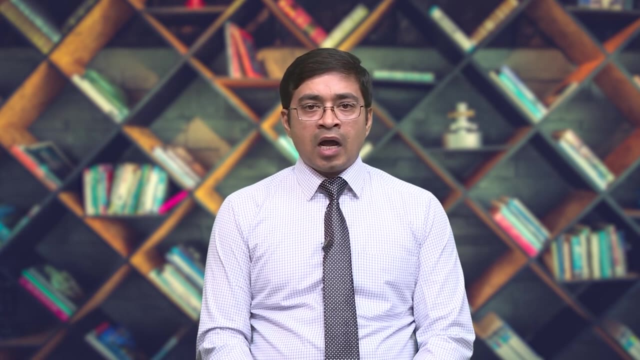 These are a graph that are not explicitly constructed and stored for any analysis Owing to their prohibitive size. Rather, they can be studied and algorithm can be run on them Based on definition of how nodes connected to one another. A simple example of an implicit graph would be a hypercube graph. 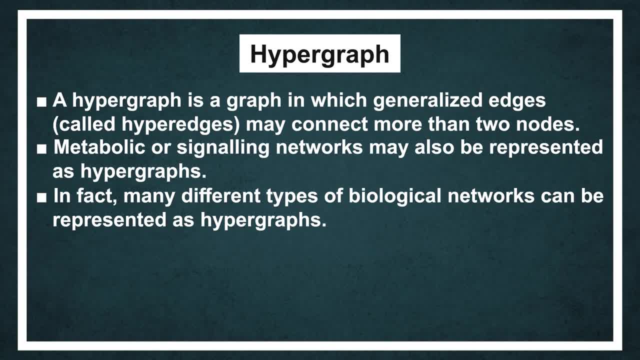 A hypercube graph in a D dimension has two D nodes With two nodes connected to one another If they vary exactly in one dimensions, For D, suppose equal to a value 3.. We have a cube with 8 nodes and 12 edges. 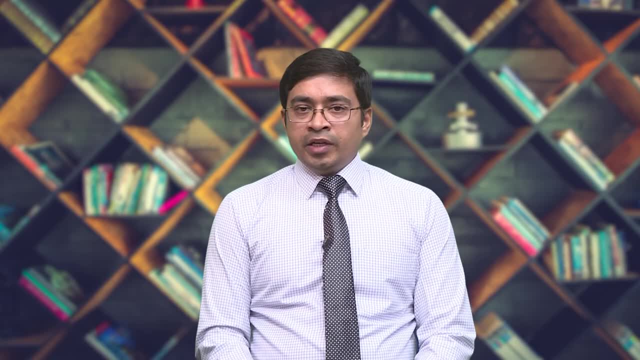 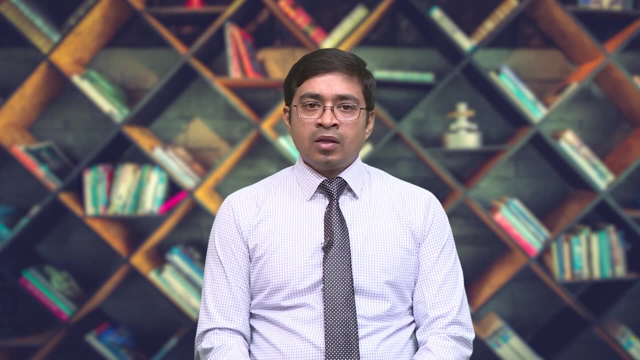 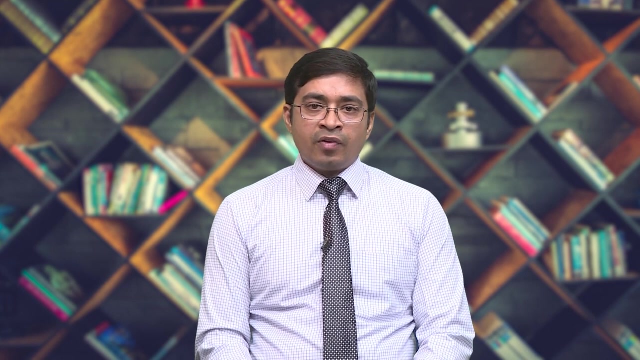 For Very large value of D. The graph will be too large to construct and to store. Yet it is possible to compute shortest path Or run another algorithm efficiently on this graph, Owing to the knowledge of the rules that define connectivity between the nodes. 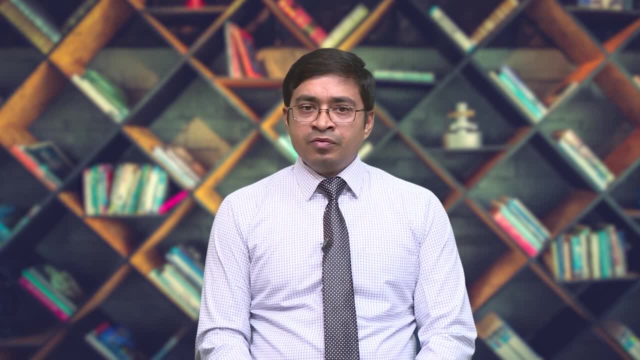 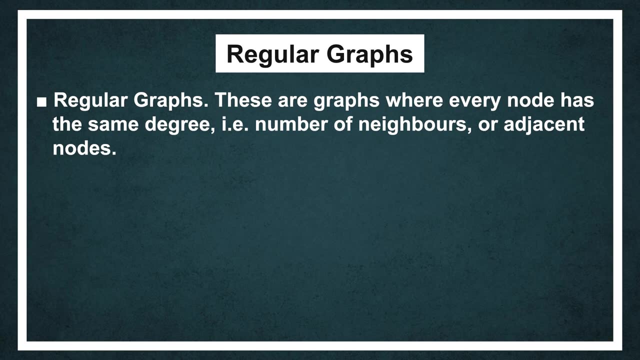 So next graph, termed as a regular graph, Which means Where every node has the same degree, For example Number of neighbors or the adjacent node Is, should be same for every vertices In expansion of this One graph, that name it complete graph. 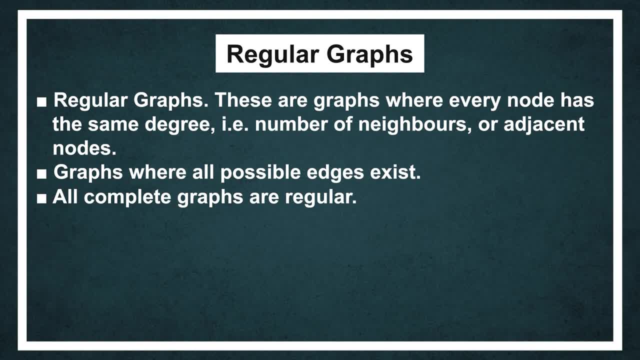 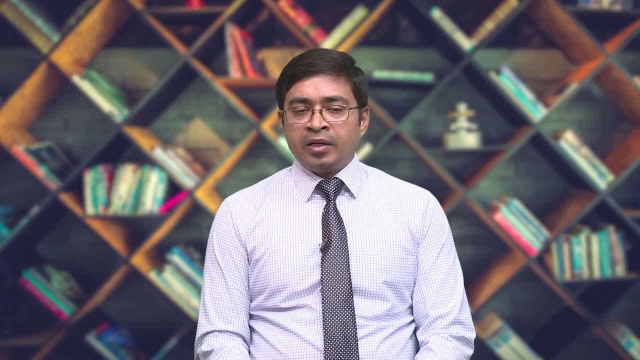 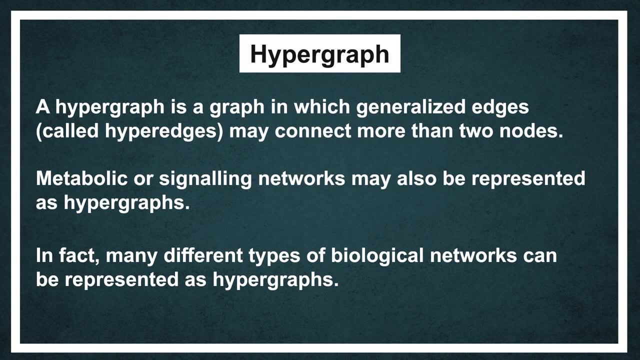 Which is all possible edges existed. All completed graph are regular. actually, The last type of graph that name hypergraph Graph typically encode only binary relationships. Often there may be any relationship among certain sets of entities. This can be better captured in hypergraphs. 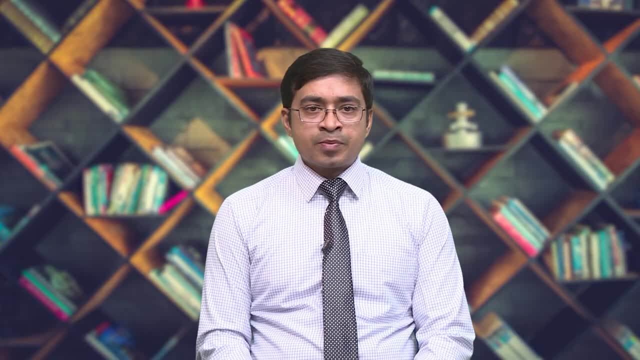 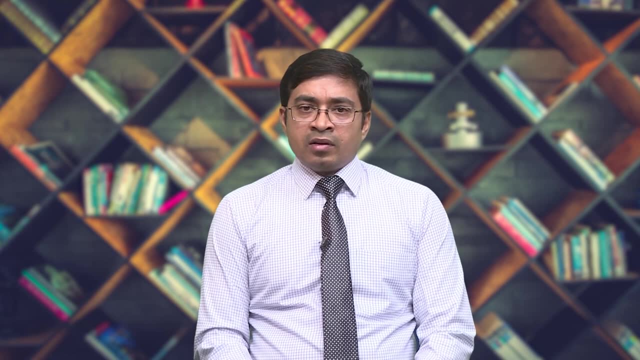 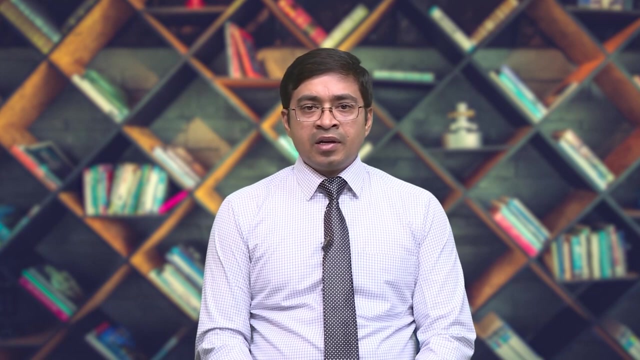 Where the set of hyper edges is not just a subset of vertices But rather than To the power V, Which means power set of vertices. In another word, Any subset of vertices can be designated as a hyper edge, For instance. For instance, 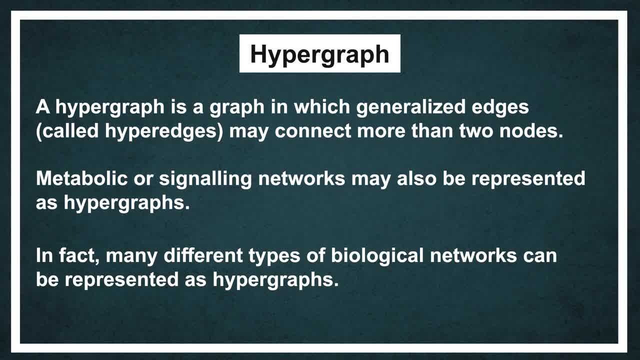 In a protein network, Protein interaction can be represented by edge. An edge between protein A and B Integrates that A complexes with B. However, If a particular protein complex contains multiple subunit, As in the case of hemoglobin, Representing them in a simple graph is very difficult. 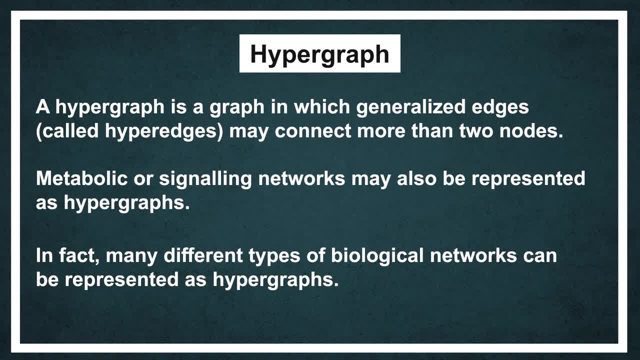 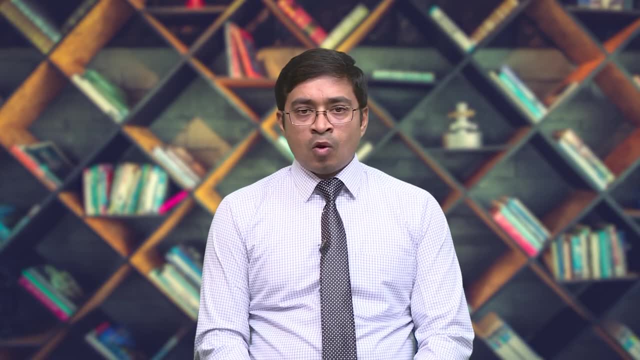 For example, G protein coupled receptor. G protein coupled receptor interact with hetero trimeric G proteins Comprising G alpha, G beta and G gamma subunits. G beta and G gamma binds to one other, make a complex Which again bind to G alpha subunit. 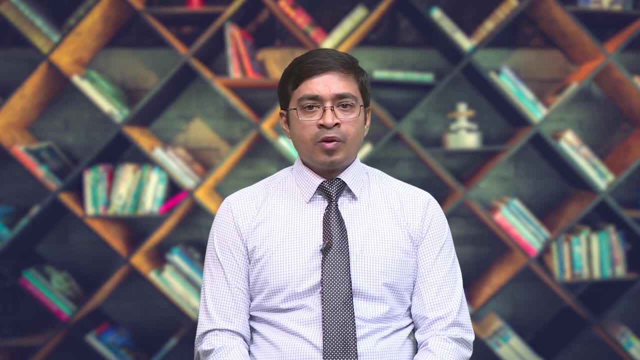 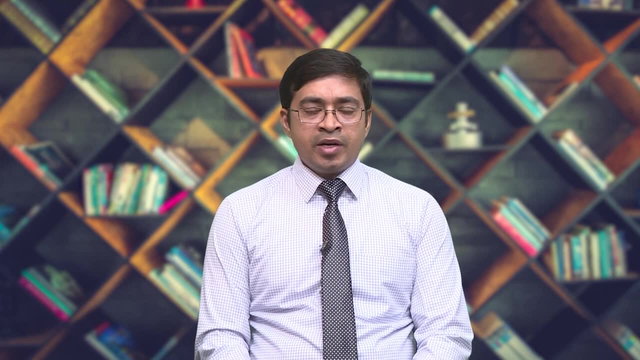 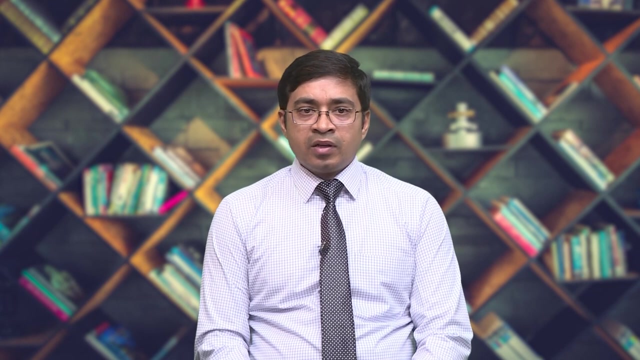 It is not possible to accurately represent this information in a simple graph. At best We would have edges between all pair of proteins: G alpha, G beta and G gamma. Metabolic or signaling network may also be represented as a hyper graph, In fact. 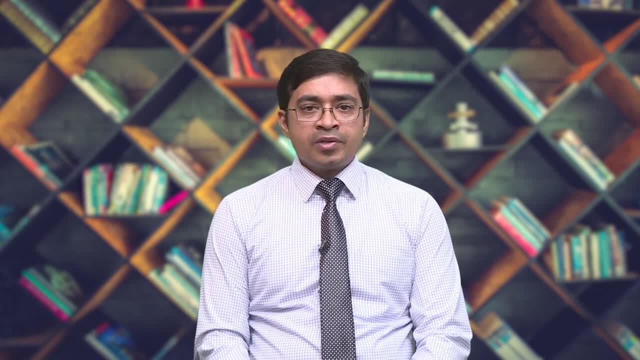 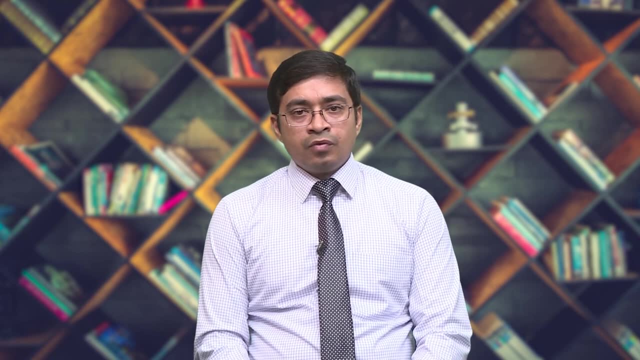 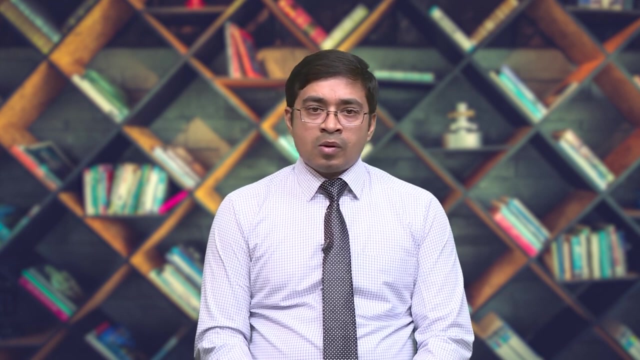 Many different type of biological network Can be represented as a hyper graph, Since the better captured any relations Vis a vis normal graph, Which typically captured only binary interactions or relationships. Now That we have a graph, We need to represent it mathematically. 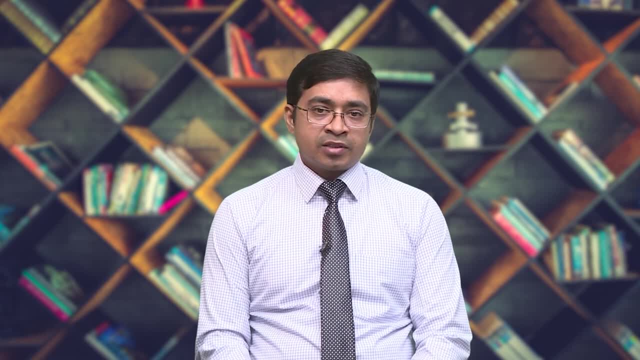 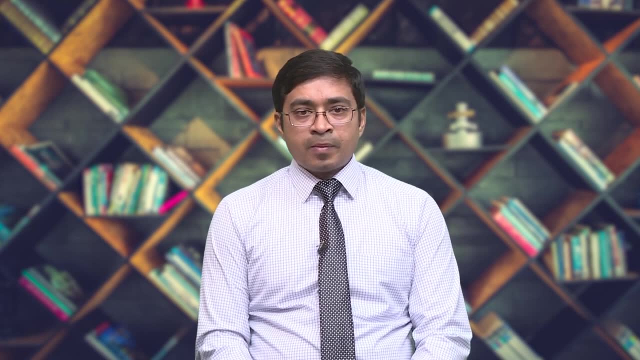 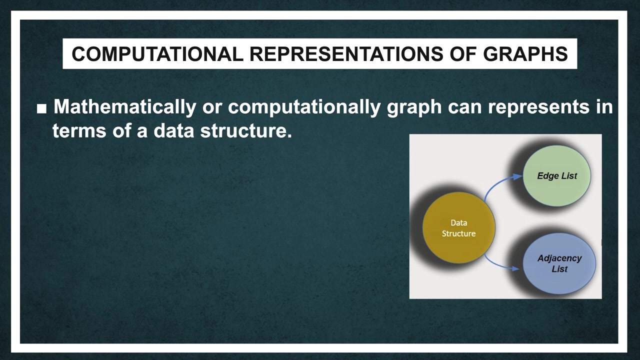 Or computationally in terms of data structure. Here we will review some basic concept of computational representation of a graph. Data structure means a number of data structure ranging from simple to efficient Are available for handling graph. Graph can be represent in term of data structure. 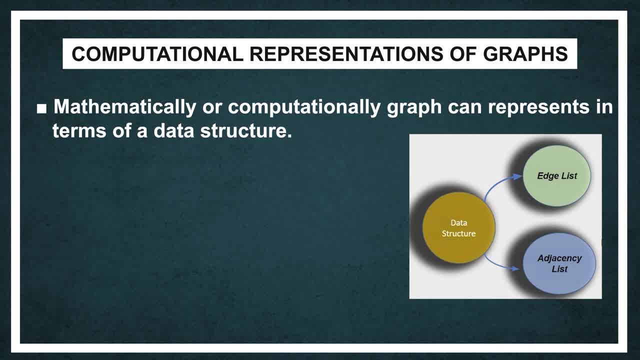 Basically, It is Comprising of two list: Age list And agency list. The age list is a simplest representation of a graph As a simple list of all ages. Although Inefficient for computations, It happens to be the easiest way to store graph in a file. 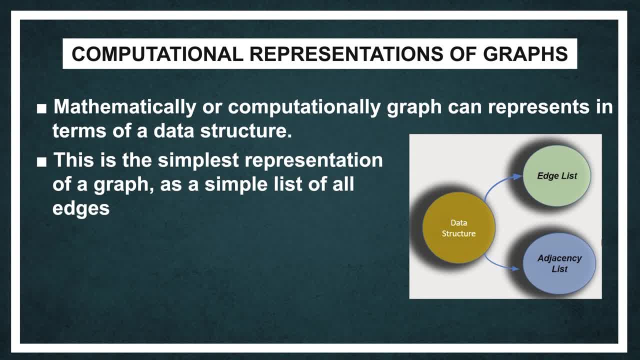 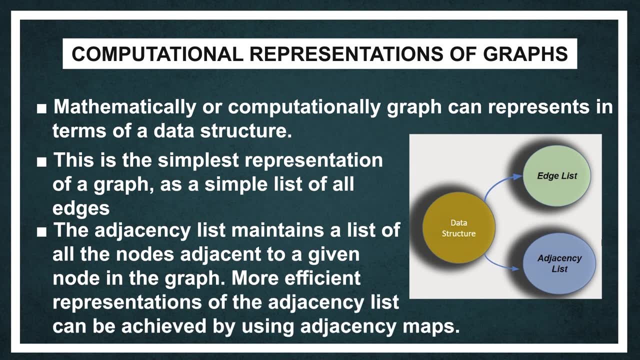 And exchange them in a human readable format. In figure C: Illustrate the age list. Illustrate the age list of the directed graph In a figure B: Agency list. This list maintain a list of all nodes adjacent to a given node in a graph. 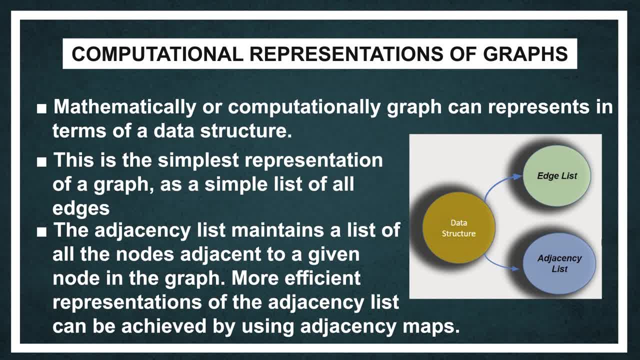 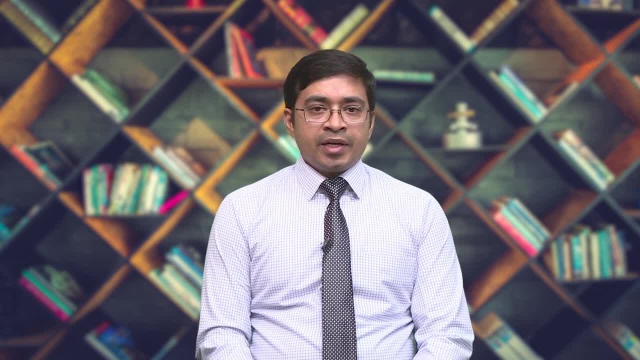 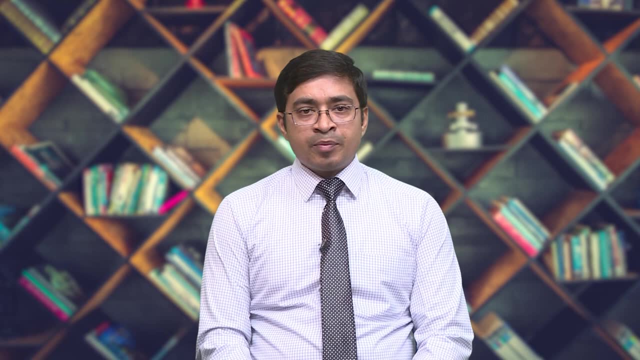 More efficient representation of agency list can be achieved by using agency map. Here, Figure D: illustrate agency list for the directed graph in figure B, Agency matrix A. very straight forward representation of graph Is the matrix representation known as agency matrix. A graph with node and edges can be represented by agency matrix. 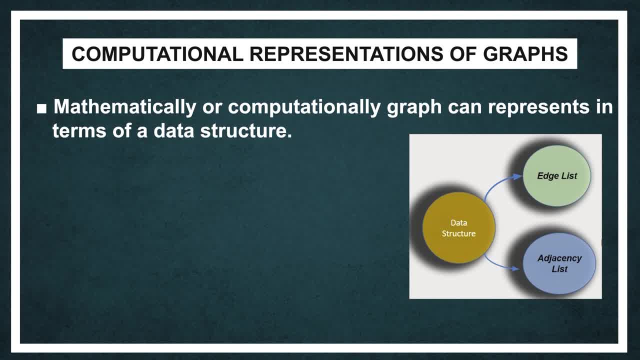 Containing non-zero entries. An entry, a ijth position in the matrix is unity If there is a edge from i to j And zero otherwise. Notably, The agency matrix corresponding to an undirected graph is a symmetric, As can also be observed from figure A. 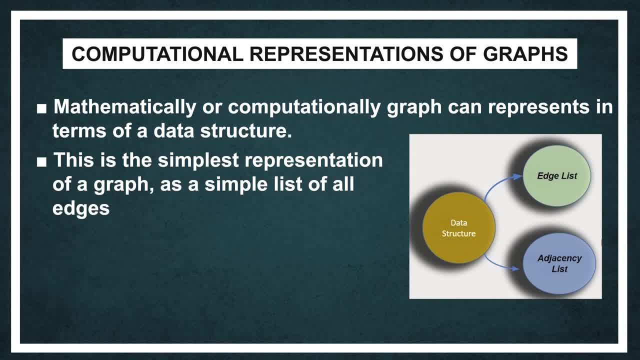 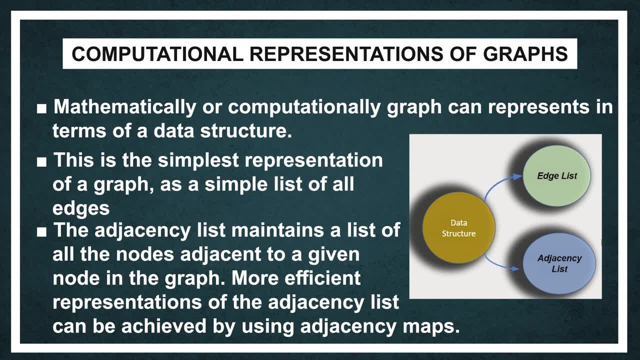 While That for a directed graph need not to be symmetric- Figure B. So To save space in practice, Agency matrix of undirected graphs can be stored as upper triangular matrix. The diagonal of the agency matrix is typically zero, Unless there are self loops. 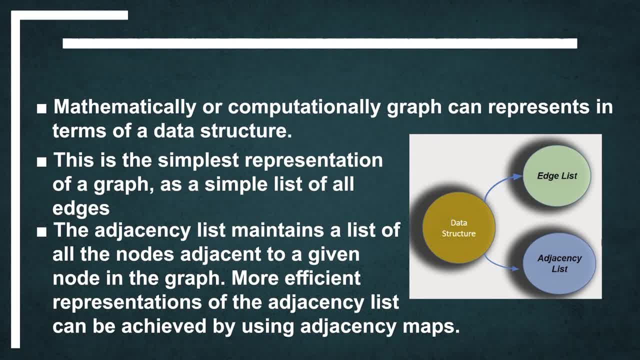 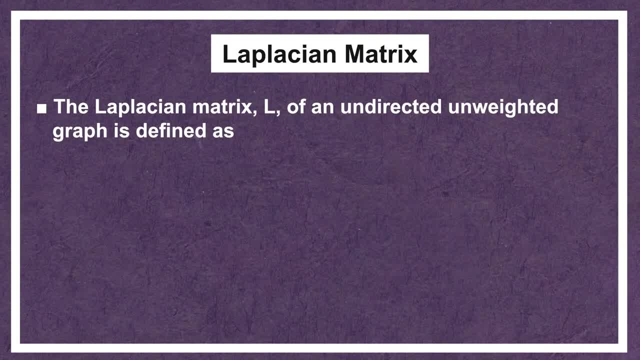 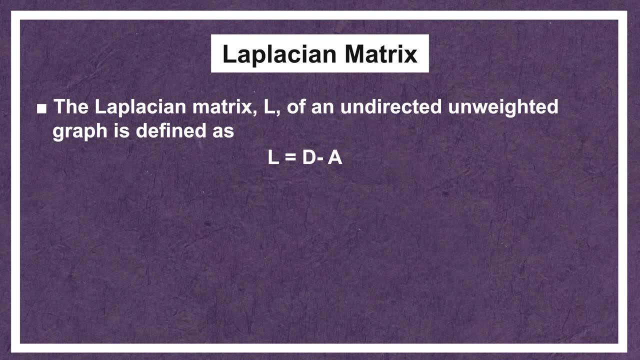 Which are uncommon in most graph. The next crucial concept is Lapsation matrix. The Lapsation matrix represented by capital letter L Of an undirected, unmetered graph is defined as L equal to D minus A, Where D represent diagonal degree matrix. 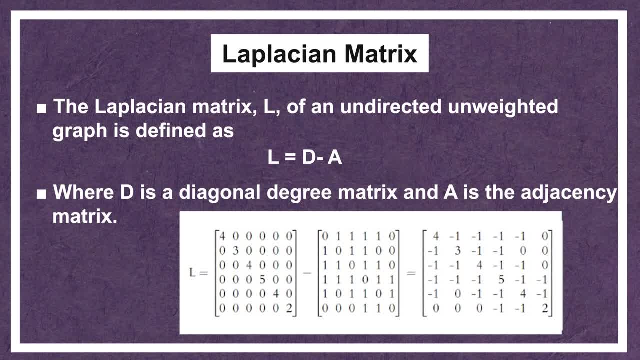 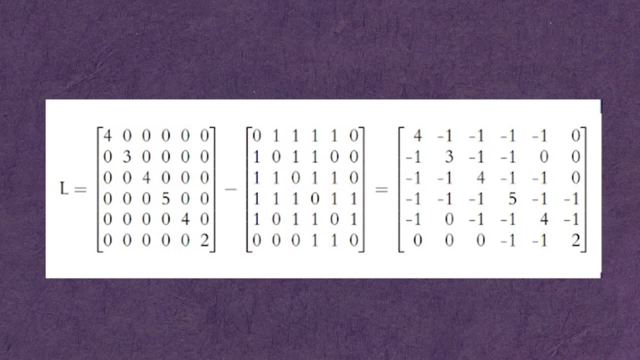 Such that D, i, ijth position Is the number of neighbors of i, And A is the adjacent matrix. If we were to ignore the weight of the graph In figure A, As provided in previous slide, Its Lapsation would be. 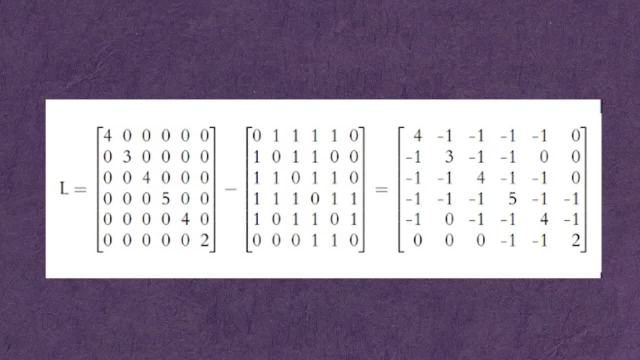 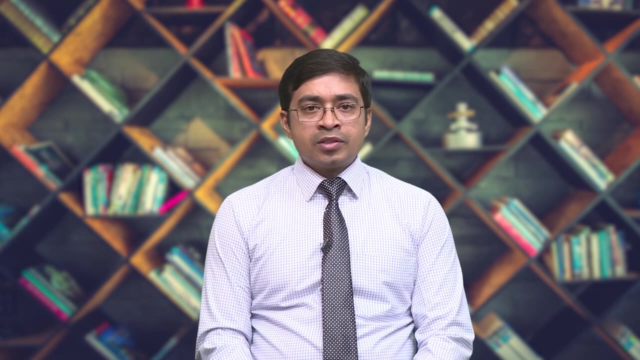 Represented in the Given slide. The Lapsation has many interesting property And is very useful for graph clustering And entry. An entry field of study, Spectral graph theory, is directed to The study of Eigen values and Eigen vectors. 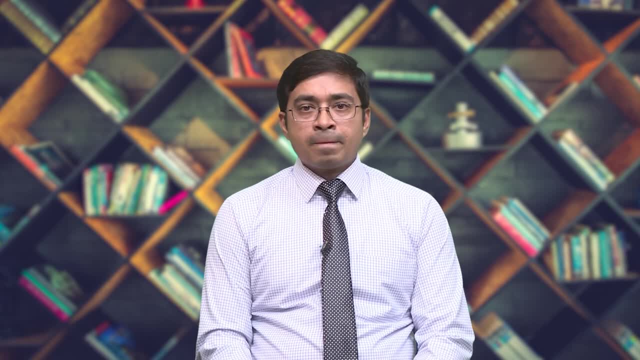 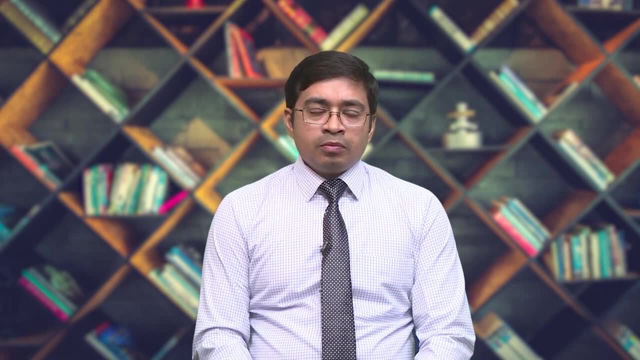 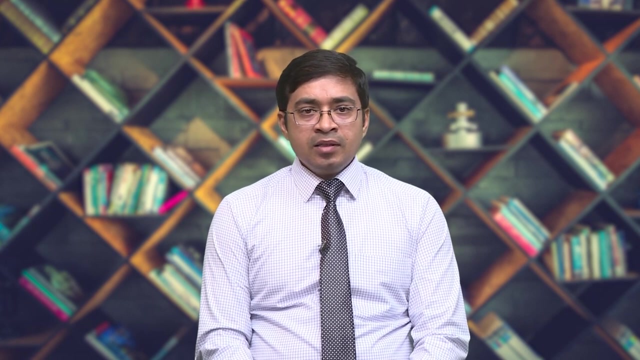 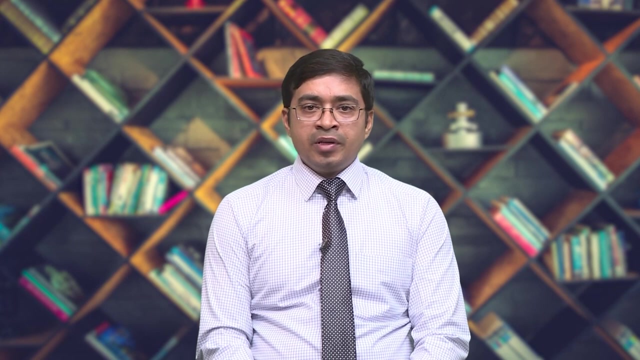 Of the Lapsation matrix. So Let discuss about the Graph representation Of biological networks. Many biological network Are naturally represented as a graph, Which also makes them Amenable to Several interesting Analysis. Here Will briefly, 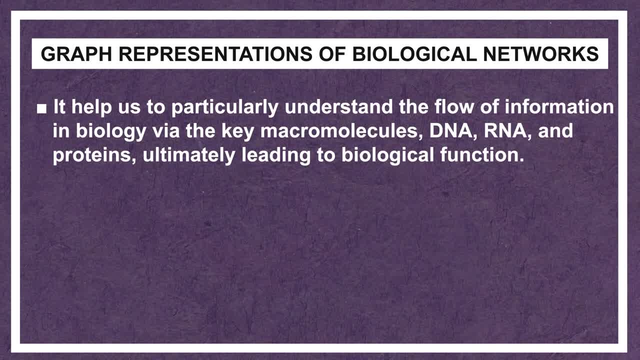 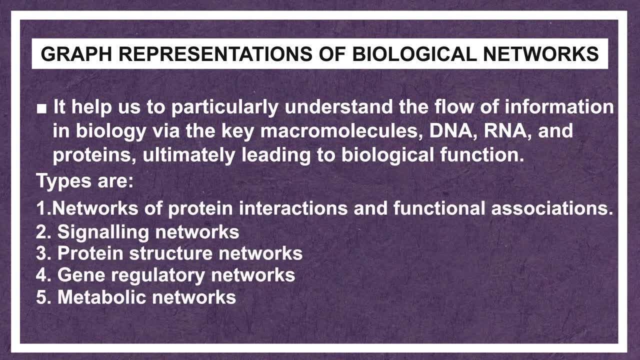 Overview Some classic Biological network And how They are typically Represented. The first Example, Network of protein interaction And functional Association Amongst The most widely studied Biological network Of protein interaction Network, As well as 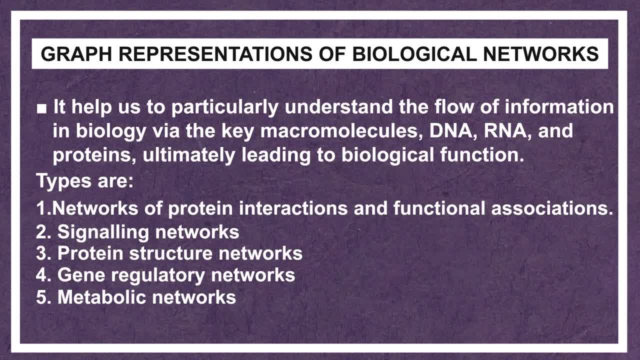 Network of functional Association. There Is The Most widely Studied. There, Popularity Is Exemplified By The Existence Of Several Database. Protein Are The Nodes Of 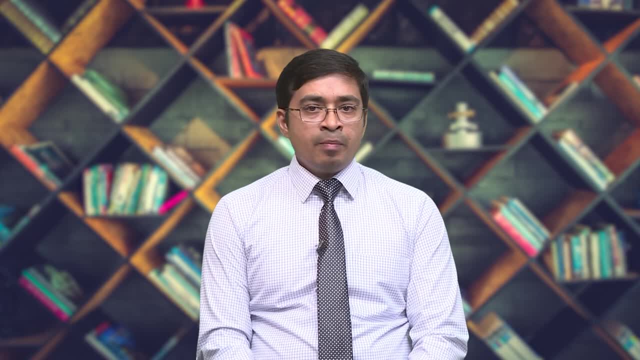 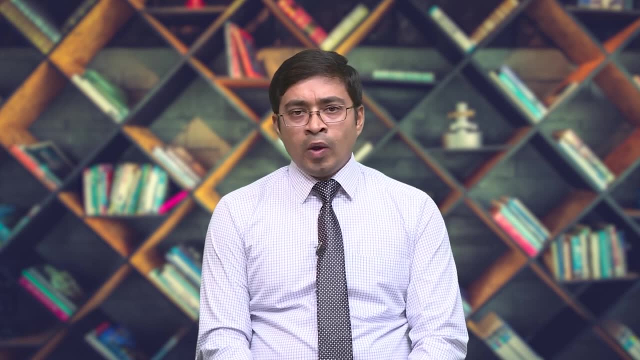 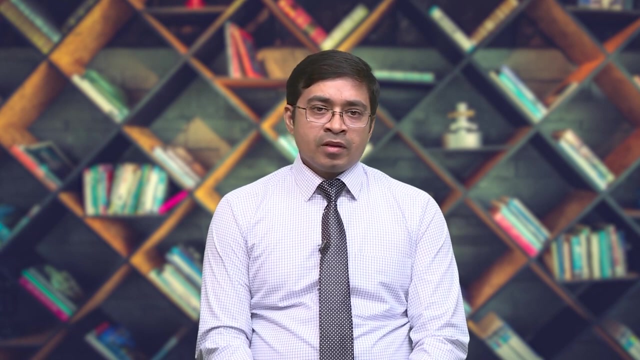 Network With Ages Representing Various Types Of Association, Ranging From Physical Interaction Complexation To Co Structural And Directed. Second Example: Signaling- Network Signaling. 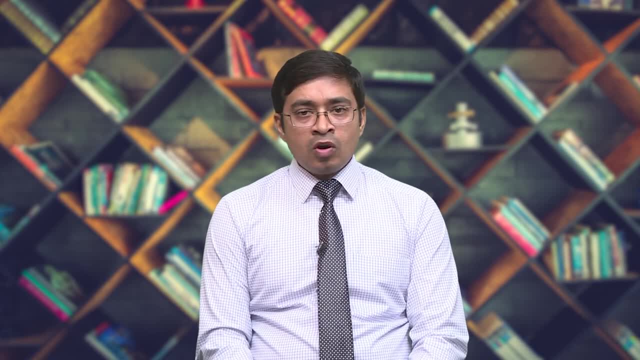 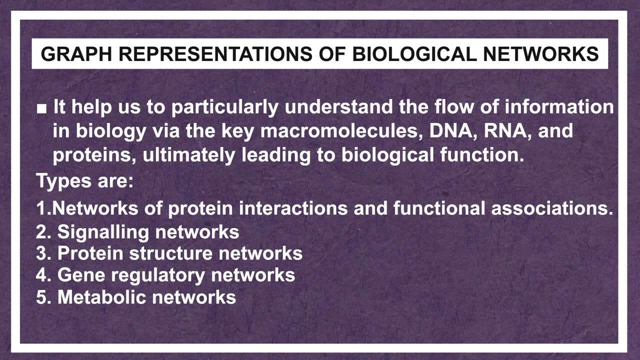 Network Comprises Different Kind Of Cellular Components, From A Receptor, Small Molecules Such As Chemical Messengers, To Intra Cellular Signaling Proteins, Structure. 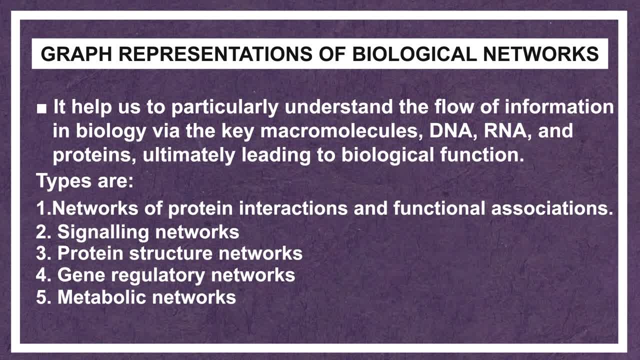 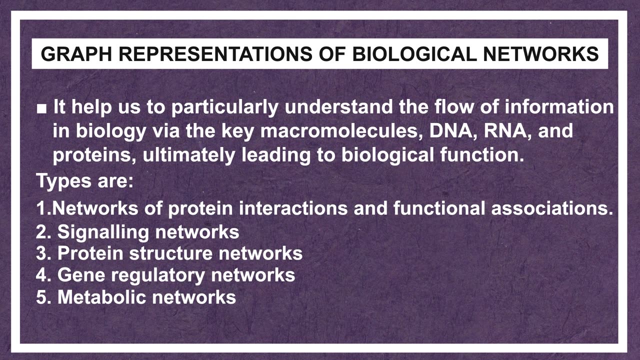 Network At A Very Different Resolution. It Is Also Possible To Represent A Single Protein As A Network Or A Graph. Many Interesting Studies Have Proposed. 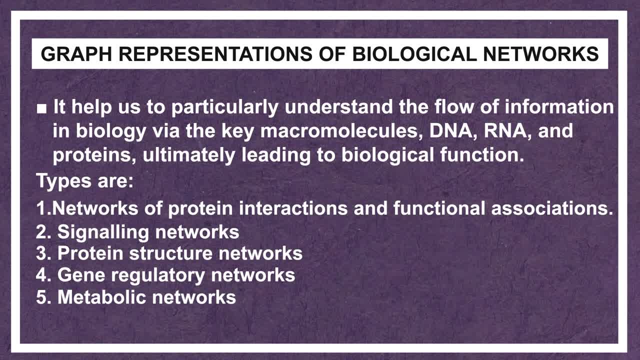 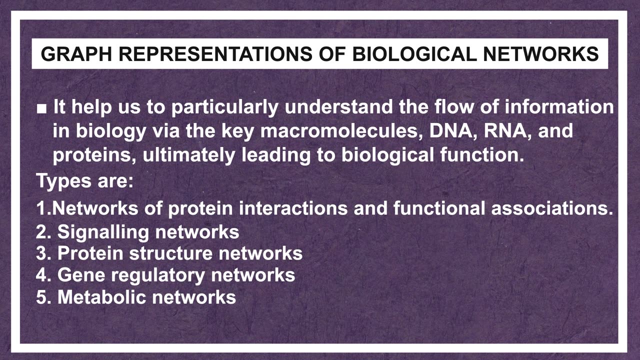 Alternate Useful That Have A Pair Wise Interaction Energy Lower Than A Particular Threshold. Fourth Type: Gene Regulatory Networks. The Reconstruction Of Gene Regulatory Network. 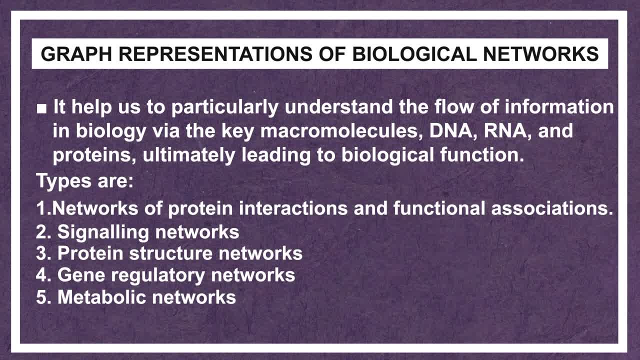 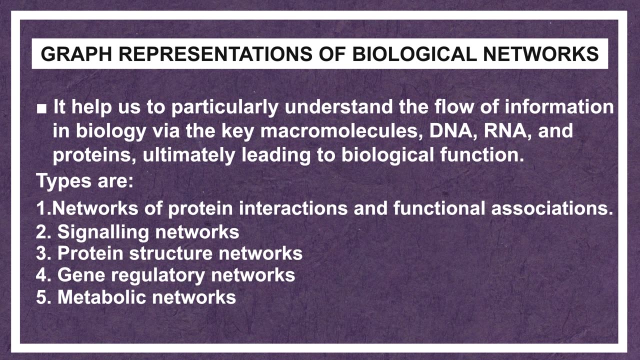 Is An Interesting Computational Challenge. Gene Can Actually Map All Interaction Between Gene And Another Genes On A Directed Graph The Age Weight Can Take. 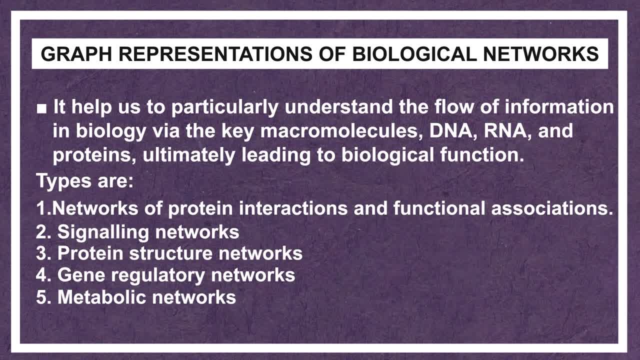 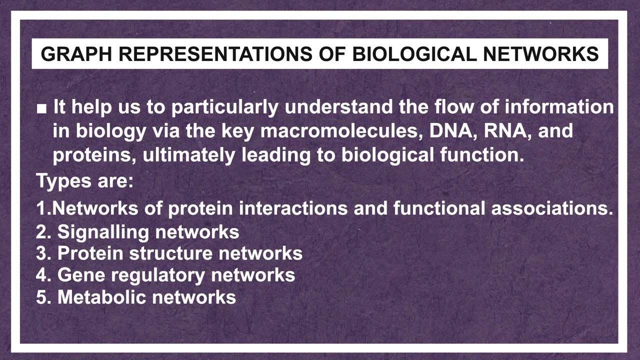 Both Positive And Negative Real Values, Depending On Activation Or Repression Metrics. It Is Also Common To Capture This Relationship In A Regulatory Strength Matrix. 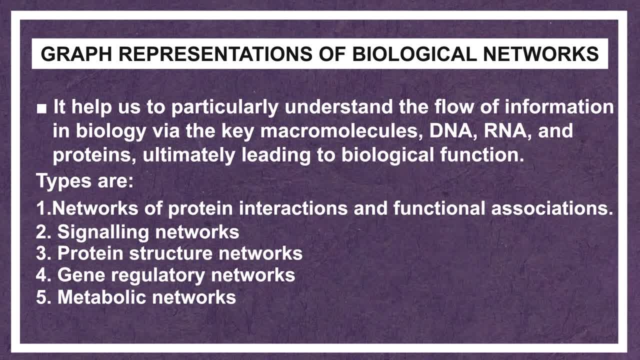 The Last Type Of Biological Network Is Metabolic Network. Metabolic Network Can Also Very Heterogeneous Map On To Graph In Various Way Presenting. 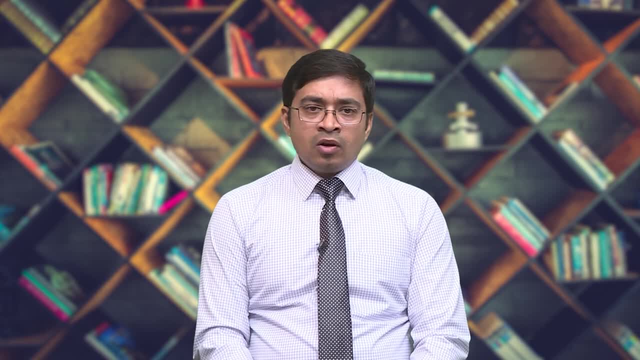 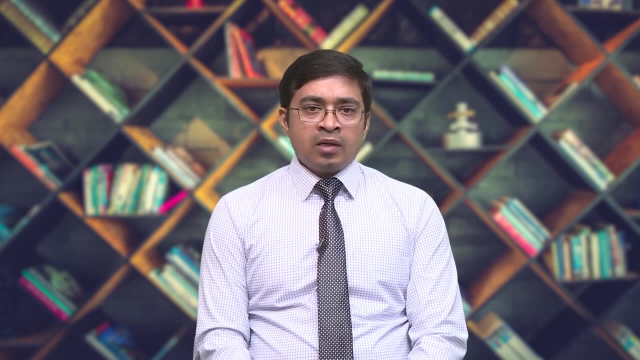 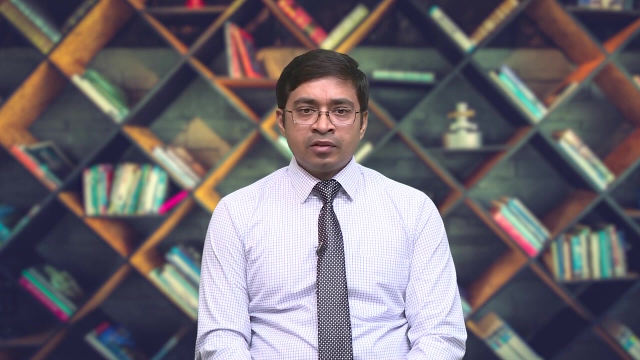 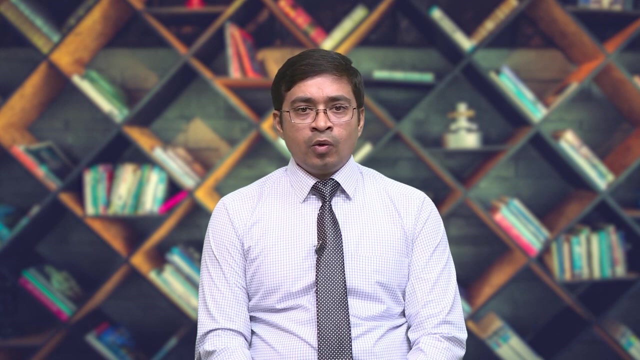 Interesting Insights Into Their Structure And Functions. So Study All Such Kind Of Graphs. There Are Several Software Tools Are Available For The Analysis And 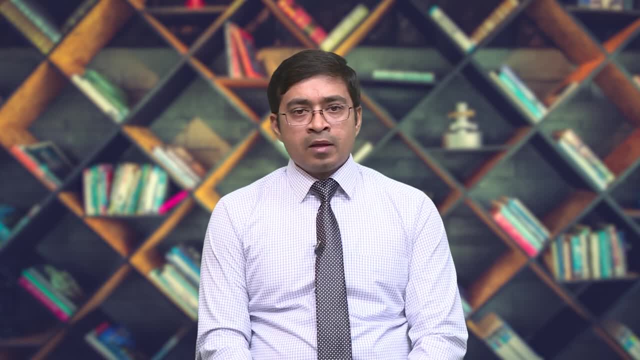 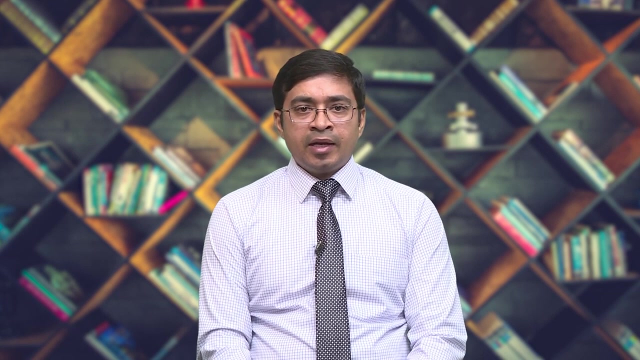 Visualization Of A Network. Notably, A Lot Of Apps Are Available For Site, Which Extends It For Various Domains Ranging From Social Network Analysis. 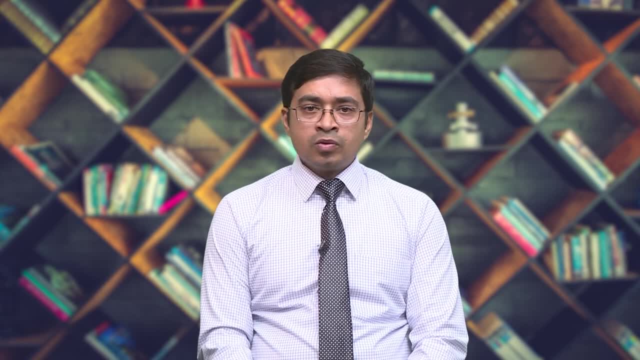 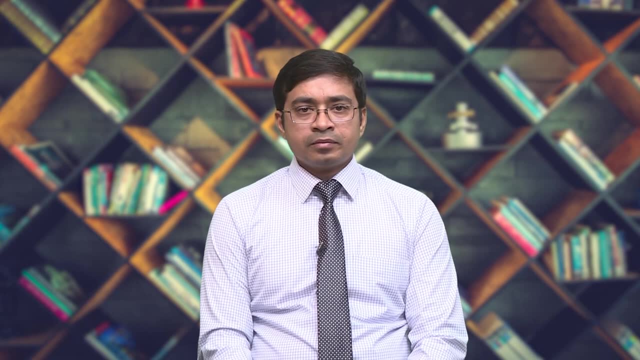 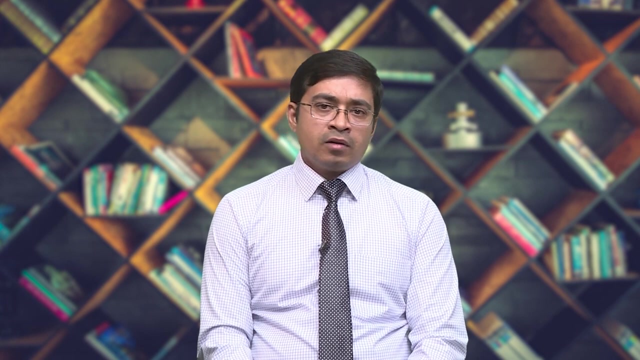 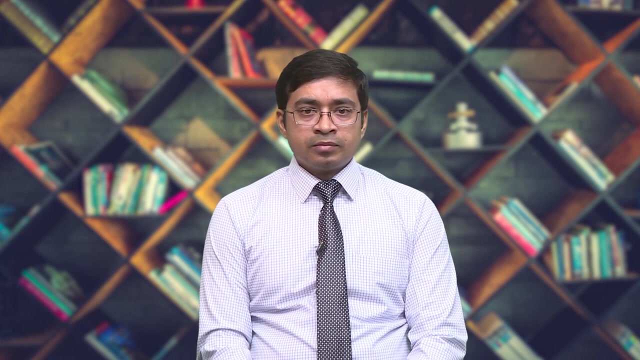 To Graph. Vis Is An Open Source Graph Visualization Software Which Many Layout Algorithm. The Fourth Is Wide Is A Free Desktop Application For Creating Various 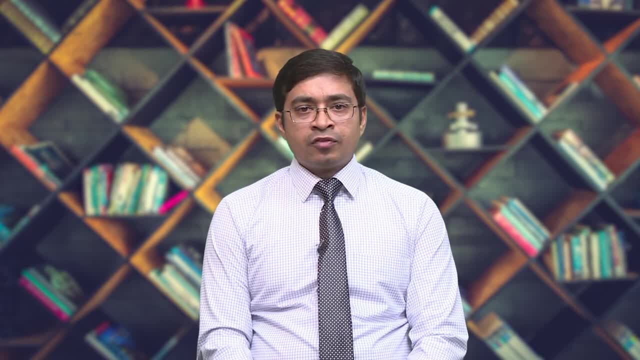 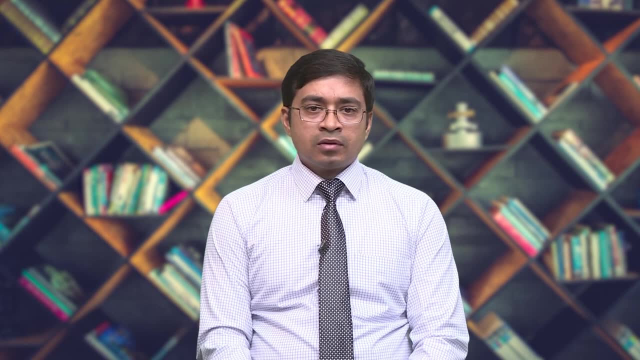 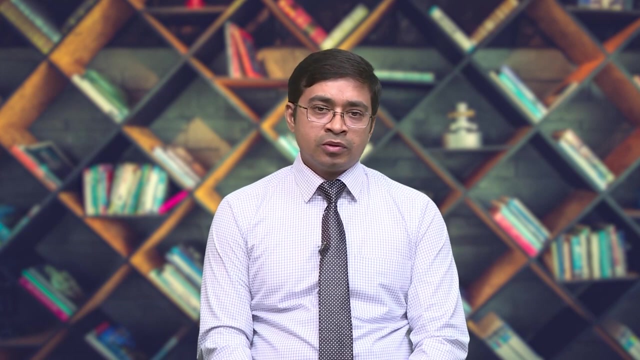 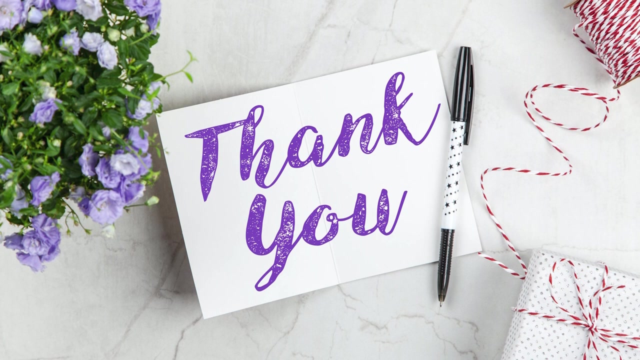 Kind Of Diagram Including Graphs To The Relevant Topic. So I Thank Everyone For Your Kind Attention. Hope This Lecture Have Been Helpful For You. Will Meet You In The Next Lecture Session. Very Soon.